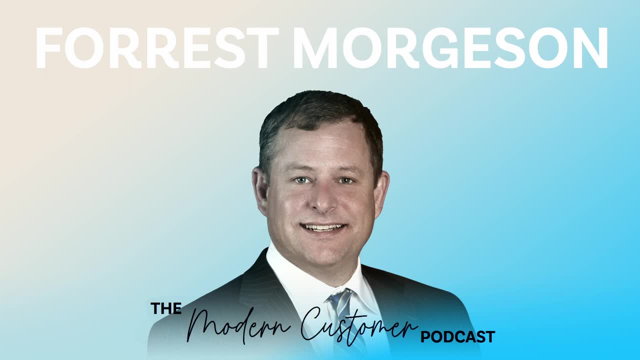 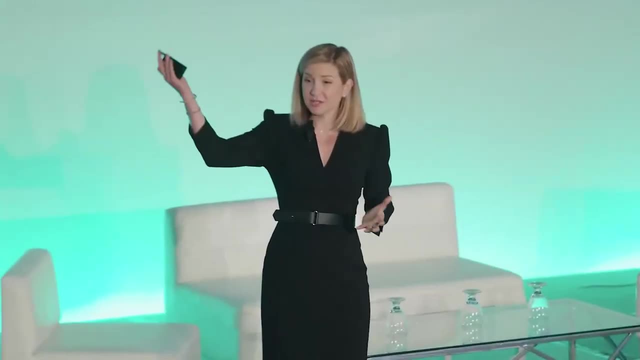 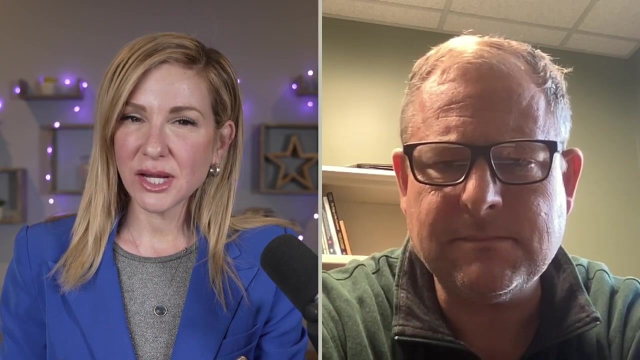 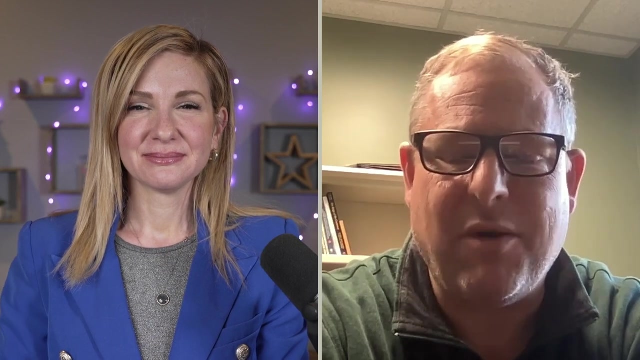 service. Please enjoy. Forrest Morgensen. Forrest, welcome to the Modern Customer Podcast. It's so nice to see you today. Welcome to the Modern Customer Podcast. I'm your host, Blake Morgan. Where are you today? I'm actually in East Lansing, Michigan, so about an hour north of my home base in. 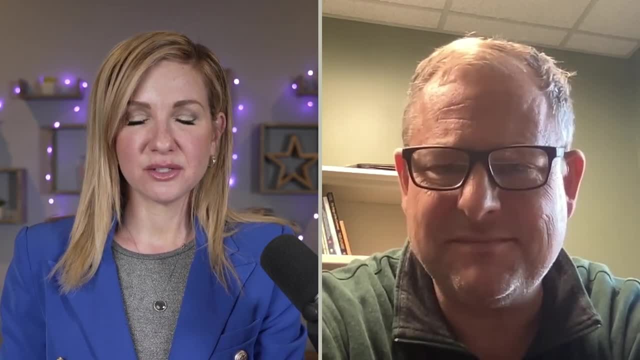 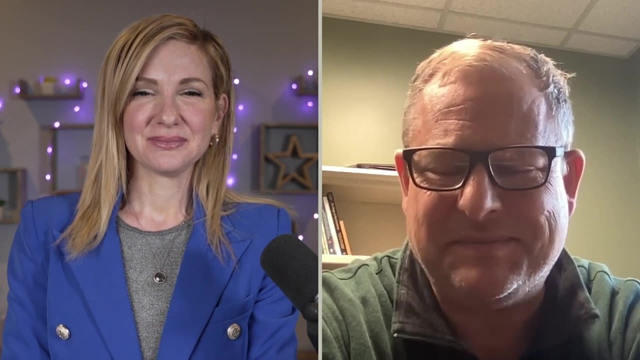 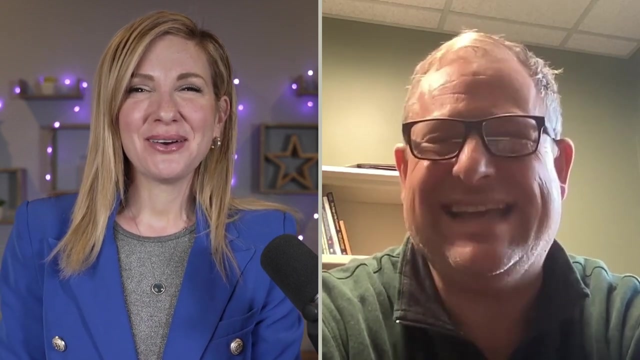 Ann Arbor, Michigan. Oh okay, Do you love living there? I hear it's beautiful It is. The winters get a little rough, but the rest of the year is quite beautiful here in Michigan. Well, yes, it's even cold here in LA today, So I'm recording with a jacket. But let's talk about you and how. 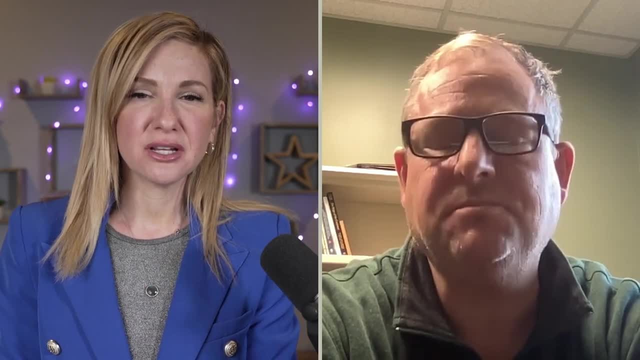 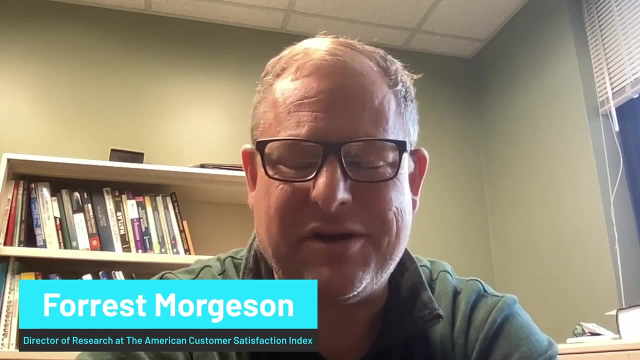 you got into customer data. Tell us the career journey and how you got to where you are now. Well, it is, at this point, a longer journey, or a pretty long journey, But I started working with the American Customer Satisfaction Index when it was still a 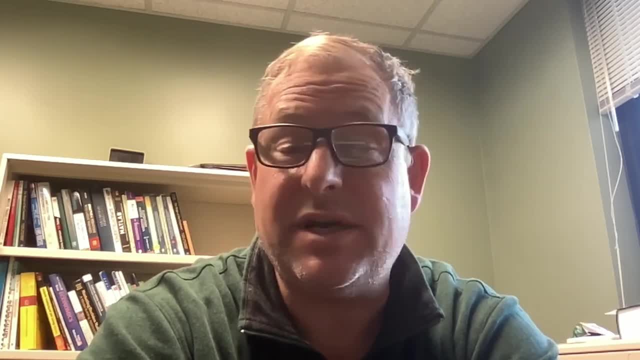 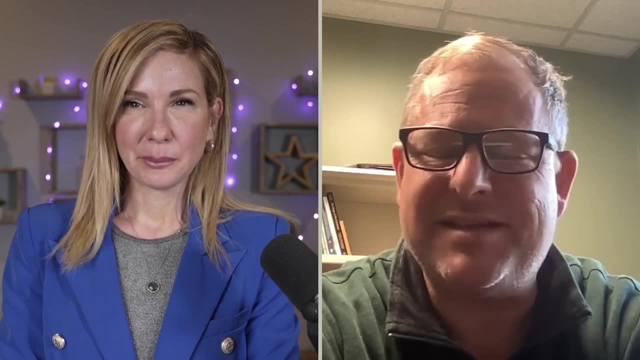 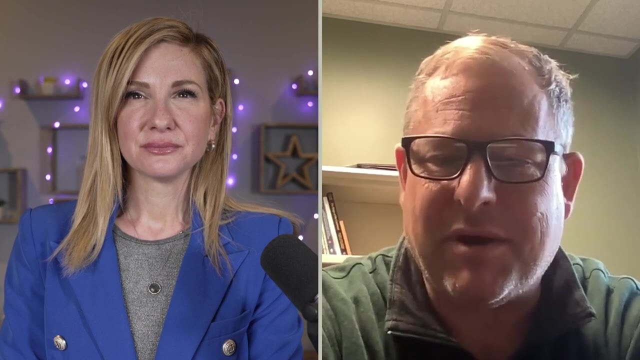 research center at the University of Michigan in 2001.. So I started working there then and have been affiliated with the ACSI ever since, Although now I'm in my primary position. I'm an Associate Professor of Marketing at Michigan State University. So down the road from Ann Arbor. 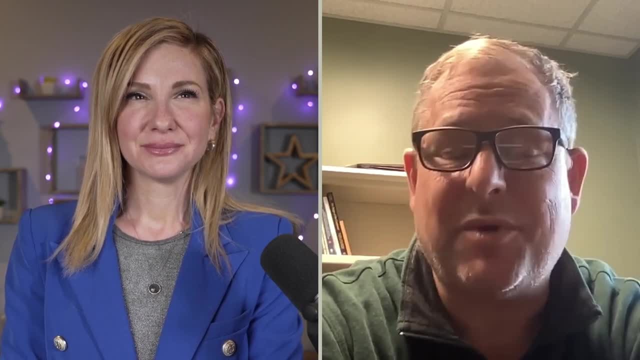 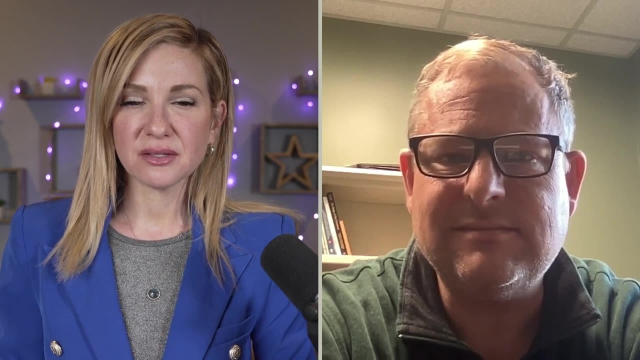 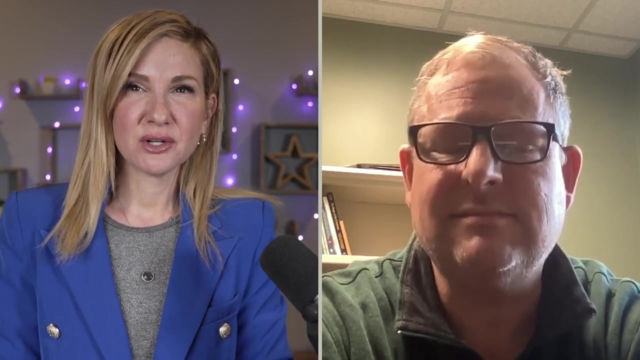 I've been working with the data for more than 20 years now. All right, So for our audience, let's step back for a minute. I recently reached out to ACSI because I was looking at the data of the state of customer service and it's not good. The customer, 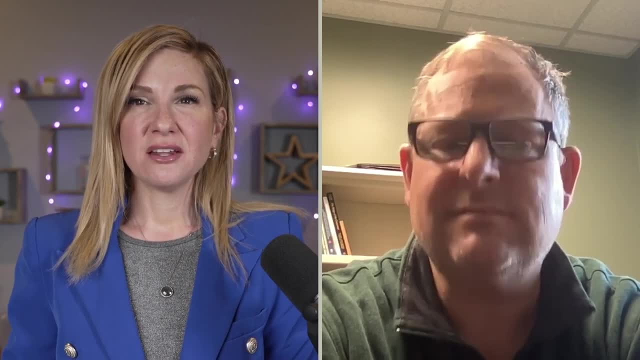 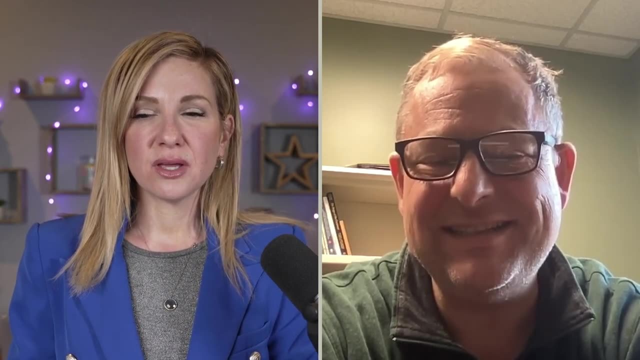 data said customer satisfaction is very, very low. And it sort of went like this: if you're watching on YouTube, just a huge dip. And then when I reached out, you know the CEO of the of ACSI said: well, it's possible, we can't even trust the data because the way companies collect 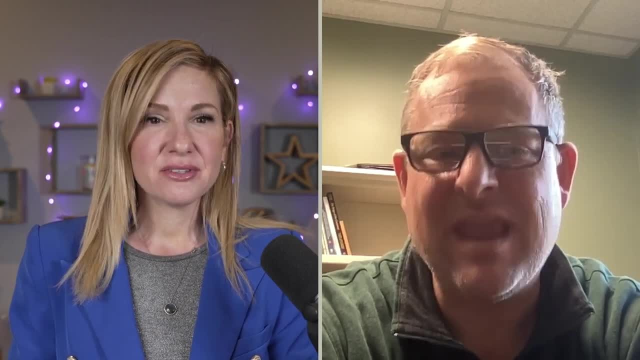 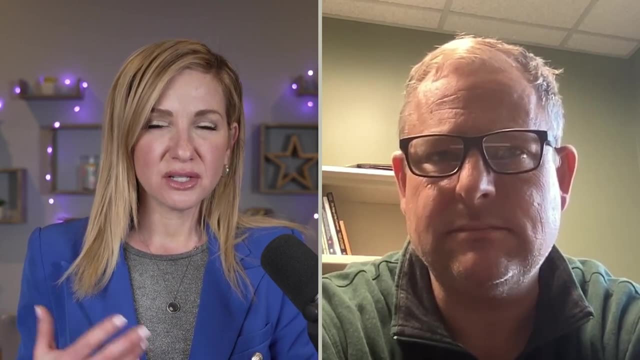 data is problematic, So I thought this is going to make such an interesting podcast. So let's just start with your view. Let's not go to the data yet, but just personally. what is your view of the state of customer service right now? It's been a really bumpy road over the last four or five. years, even before COVID hit. So a solid two years before COVID hit, we started to see a downturn in customer service. There's, I think, a variety of different explanations for that downturn. I think some of it has to do with the way that we're measuring and trying to understand customer. 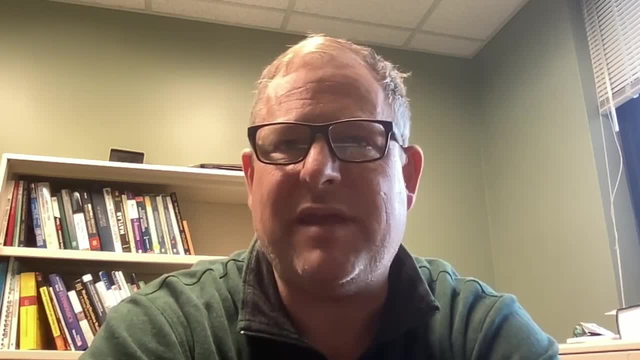 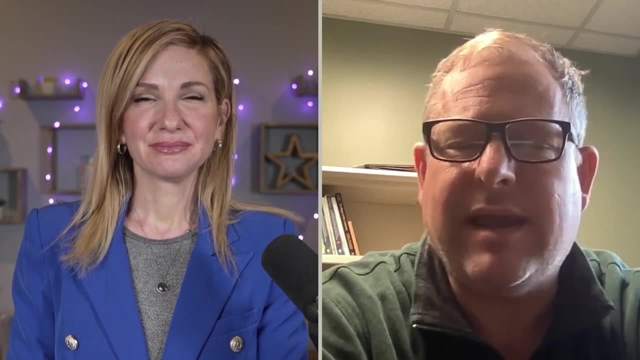 service. We still have some deficiencies in the way that we do that within organizations. We're also measuring. our companies are measuring their customer experiences in different ways and they're still getting their feet under them in terms of how they do that measurement. 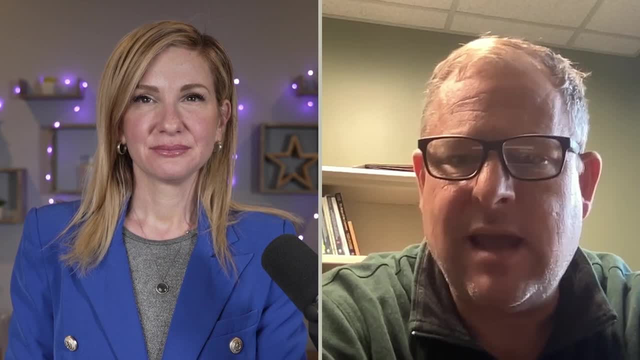 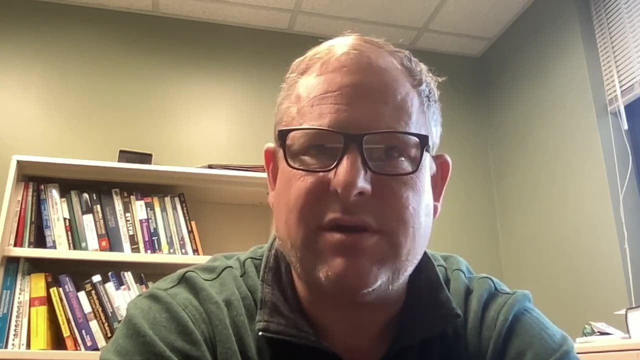 focusing more on social media and those kinds of things. And alongside that, of course, you know you have companies that sort of to some extent participate in a little bit of a vicious circle where their customer satisfaction and customer service improves, improves, improves, and they 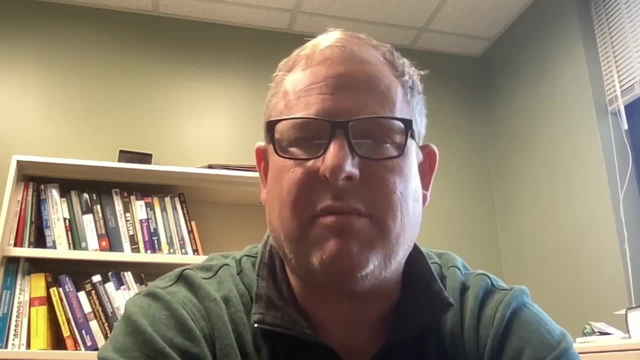 see the benefits of that in terms of stronger relationships with customers and then try to take as much profit as they can be as profitable as they can. and then try to take as much profit as they can be as profitable as they can. and then try to take as much profit as they can be as. 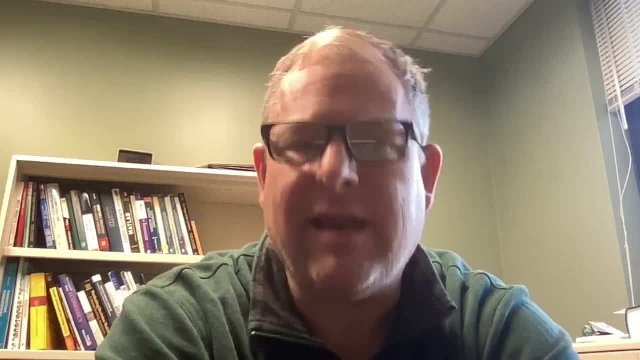 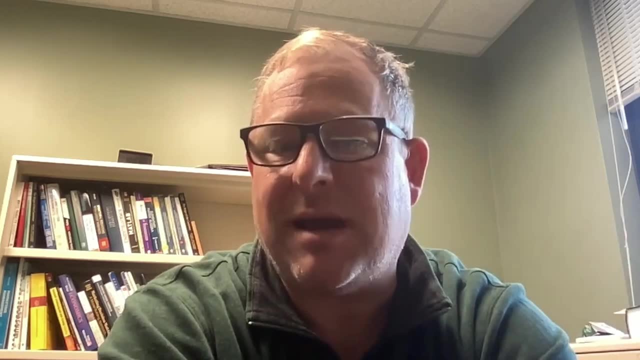 profitable as they can for their shareholders. and sometimes that will involve cutting, you know, cutting those customer services in the places where they're doing well and they justify that by saying: but we're doing such a good job with our customers that we can afford to do a. 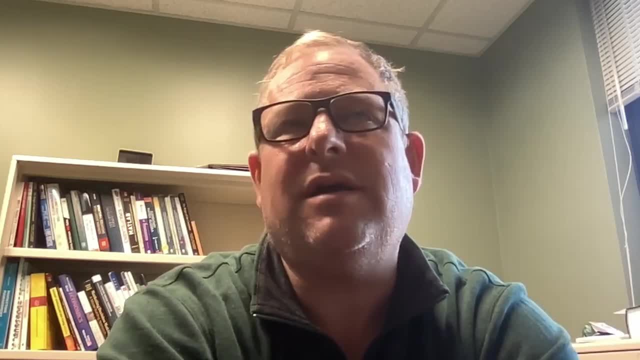 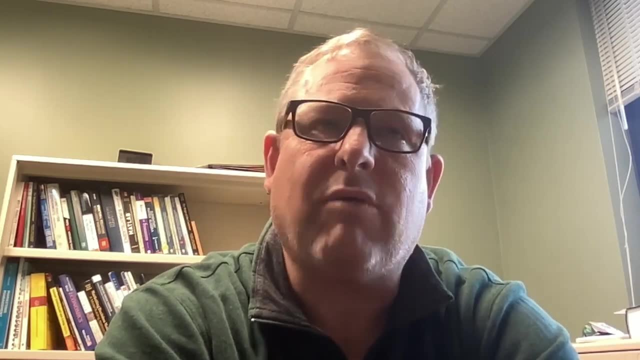 little bit less now. Regardless, we saw sort of a downward trajectory a couple of years before COVID hit, and then that was really exasperated by the arrival of COVID and all of the restrictions that that placed on the economy, And then, of course, in the wake of COVID, as it started to wean. we had the huge uptick in inflation, which had a big impact on how customers perceive not just the prices but the value that they're getting from different service providers and the products that they're purchasing. So we've had sort of a pretty significant downturn over the last five. 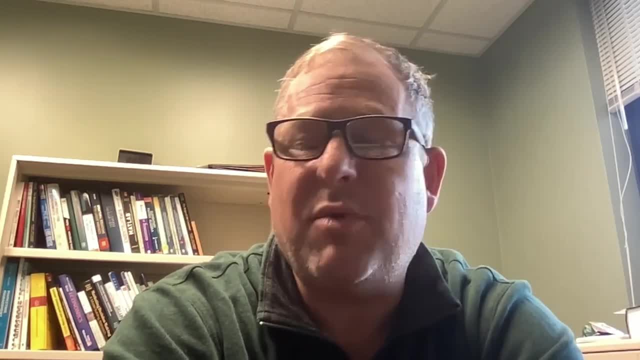 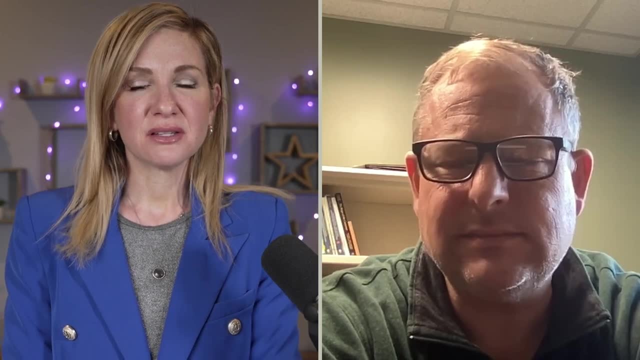 years, you know, caused by interrelated but in some ways very separate phenomena that have all weighed heavily on the economy. Yeah, absolutely. I mean, it's definitely a very uncertain time and companies seem to be just pulling away. I believe Forrester said that they're not investing in. 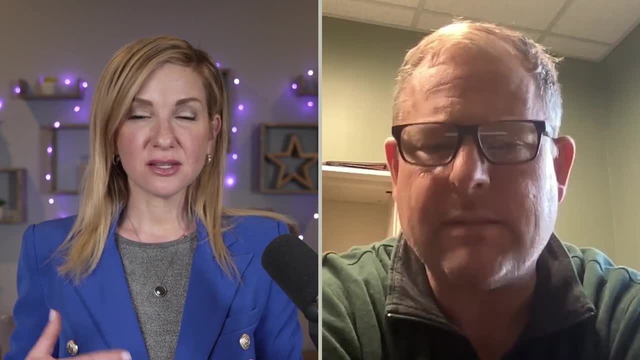 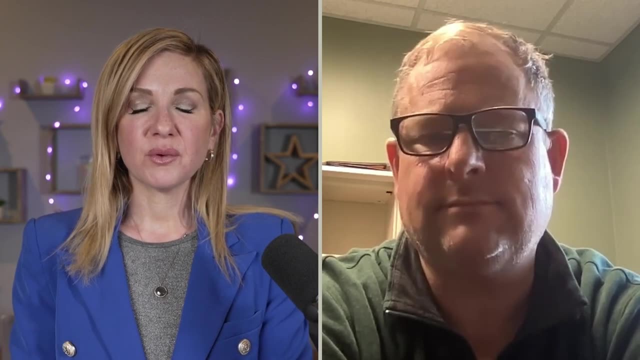 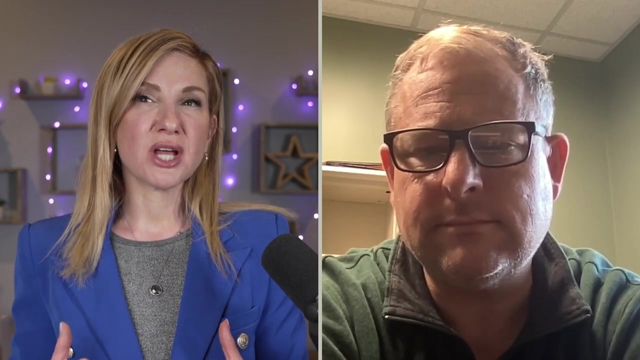 customer service because they're tired from COVID. because they extended themselves, They overextended themselves for their customers. They're tired. They want to invest in other programs. When I had originally reached out to ACSI and looked at the data, the CEO said there were some challenges. 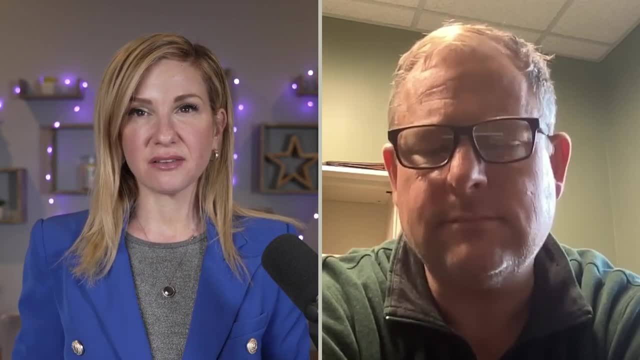 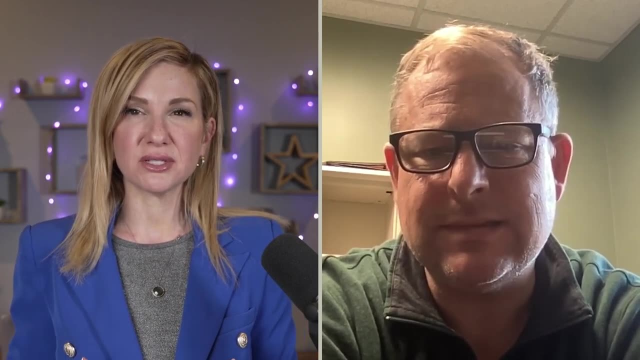 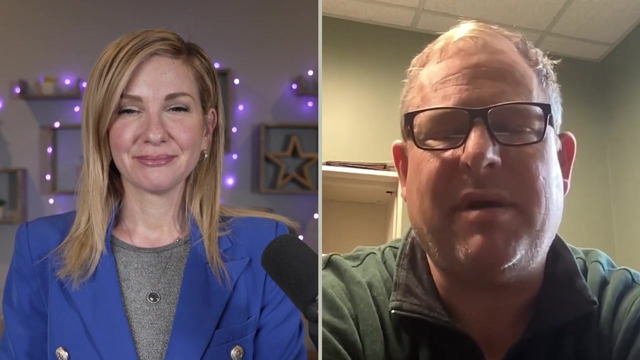 and problems with the data, the actual data of how customer satisfaction is collected. Do you have any thoughts about that? If there's a problematic process to how companies collect customer sat data today, Well, I mean, there's a variety of different challenges that companies are facing. And now 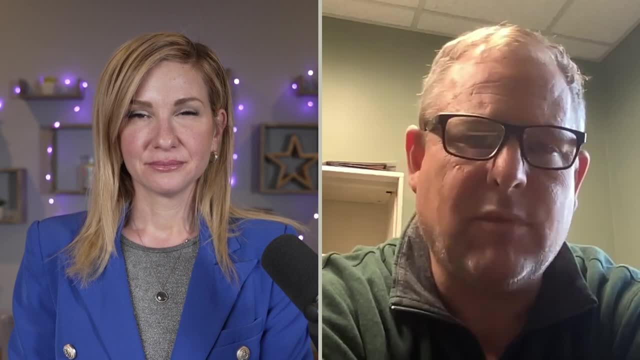 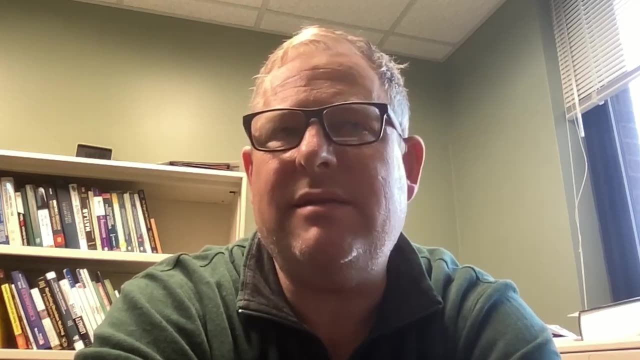 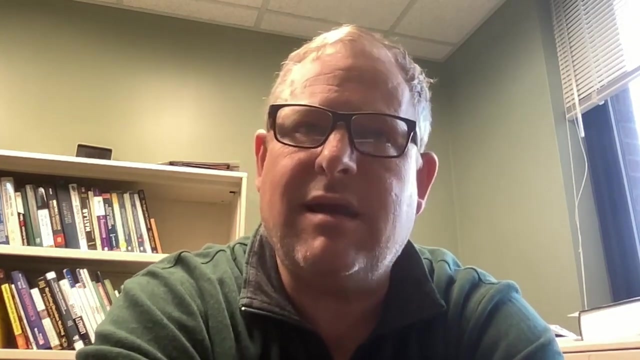 I'm talking about how the broader corporate landscape looks at and measures these kinds of things. First and foremost, one of the big problems is that we still do this, in many cases through traditional customer surveying, And that's a, you know, a strong and reliable way of collecting data into these kinds of consumer experiences. 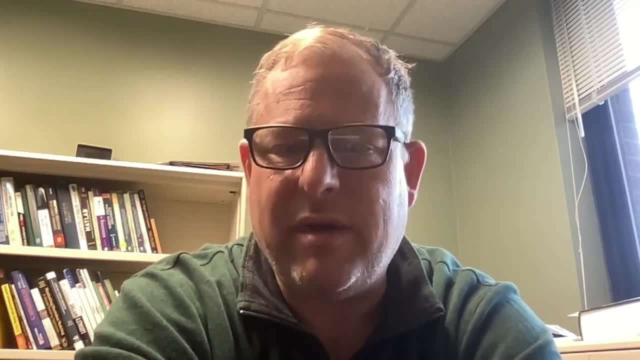 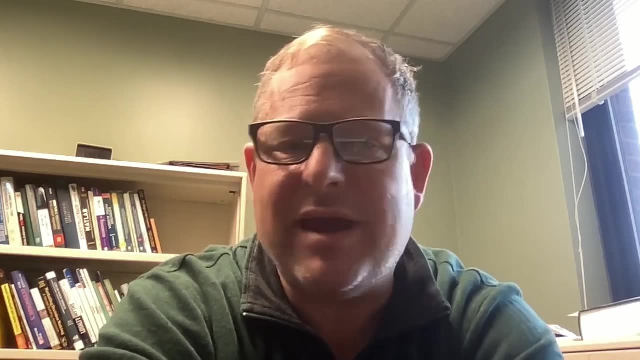 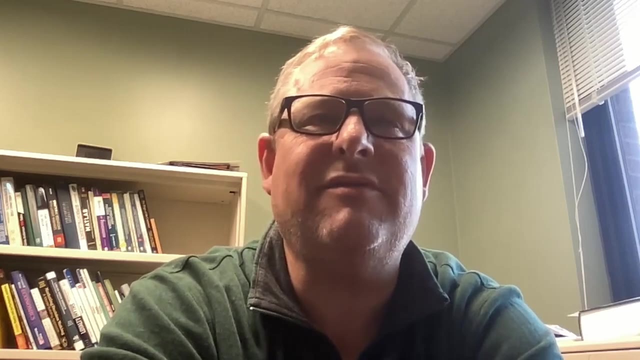 The problematic part is that we, as consumers, are more inundated with those kinds of surveys than we've ever been before, whether it's the SMS survey requests that you get just after you leave a retailer, or the email that you get, or still we get phone calls and these other kinds of methods. to try to get us to respond to customer surveys. We get more of those than we ever did before, And what that ends up resulting in is a whole lot of consumers that don't want to take these kinds of surveys, And that gives us samples of data that aren't necessarily representative of the population. That's part of the problem, And we still see, I think, too much in the corporate landscape sort of attaching our customer experience metrics programs to unreliable methods of collecting this data. 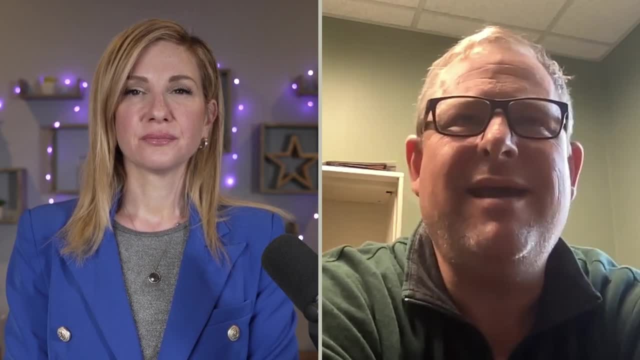 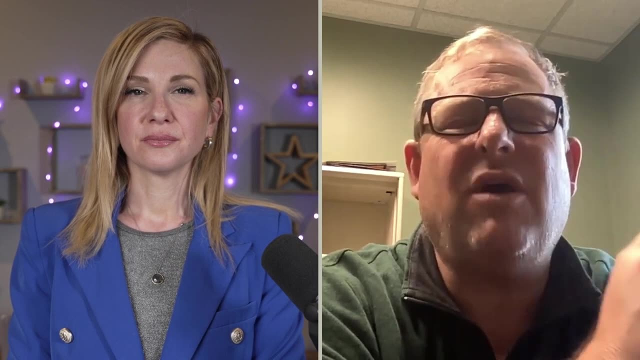 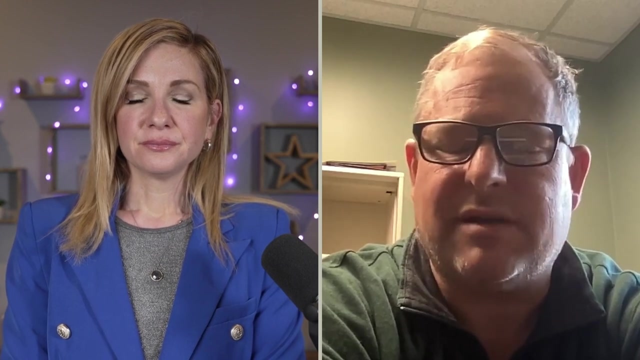 There's too many fads in the marketplace, too many, you know, quick fix kinds of methods that companies still use to measure consumer experiences that don't really allow for reliable data that gives us valid insights into how to improve our customer services. So the surveys are problematic. Customers don't want to take surveys. I never, ever, take surveys. 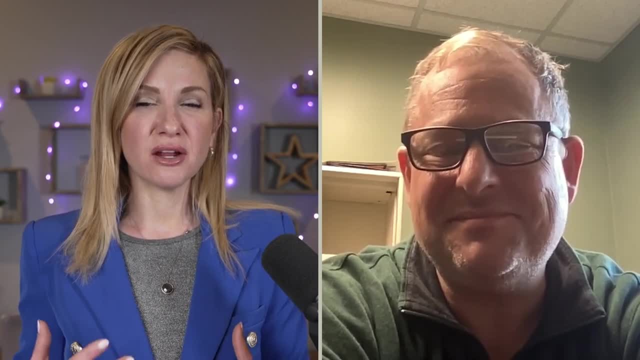 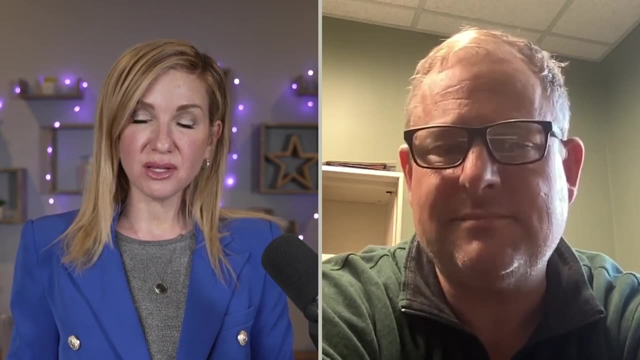 And the companies. just it seems like aren't advanced or sophisticated enough now to measure Grab data, unstructured data, and comb through it, even though the technology seems to be there to be able to see if a customer was happy or not. 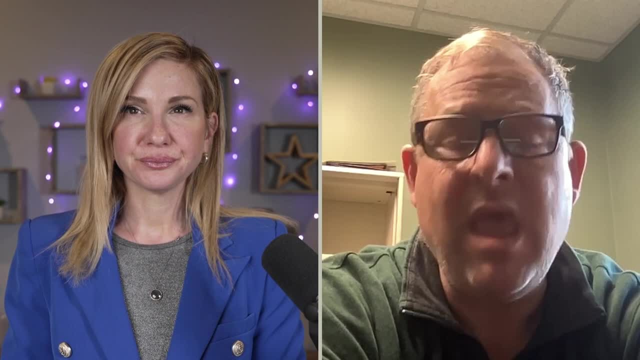 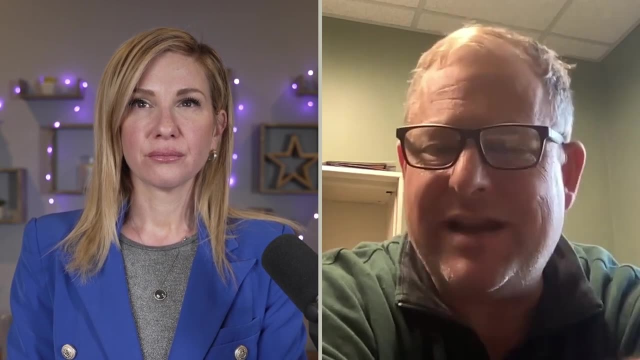 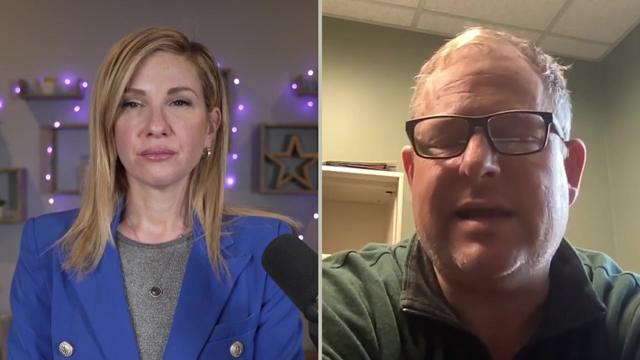 But somehow there's some kind of gap there. Well, I mean, you know, there's a big range in the quality at which different companies and different industries measure and analyze this data. There are certain industries that have adopted really, you know, sound, advanced techniques for gauging their customers' experiences and their satisfaction with data. 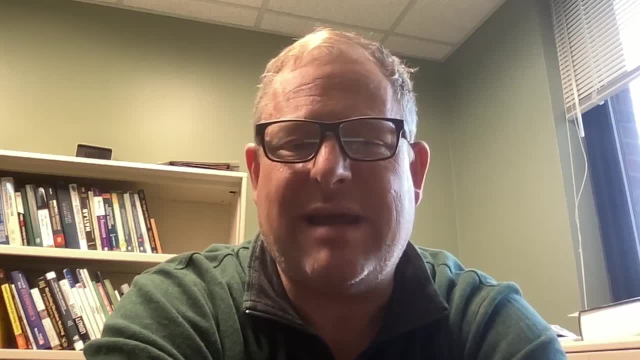 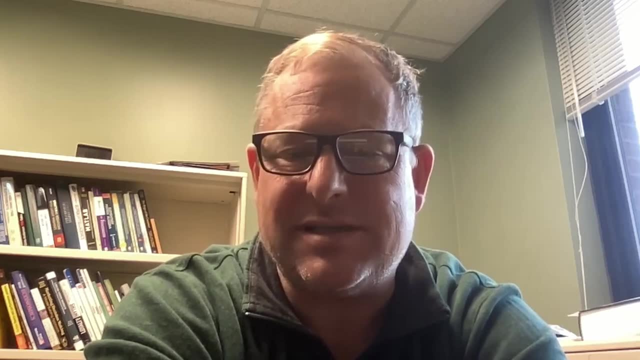 Goods and services, And there's others where they just haven't invested the time and the resources into doing that. And so you know, I think, to be fair, it's important to say that there are really wide differences across companies and industries on how well they do this sort of thing. 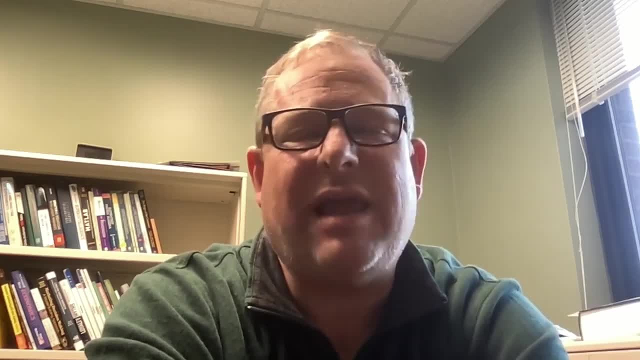 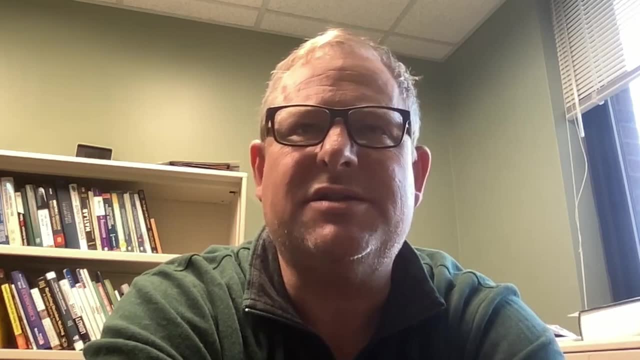 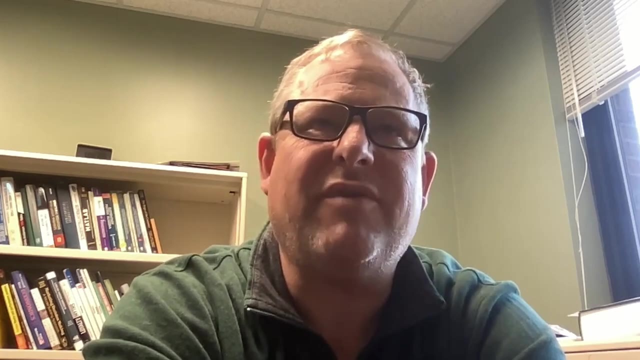 They're not all terrible at it. That being said, you still see reliance on too many metrics that are questionable, sources of data that are questionable, The view of market research and consumer experience research as PR more than as process improvement. That is still pretty prolific across industries. 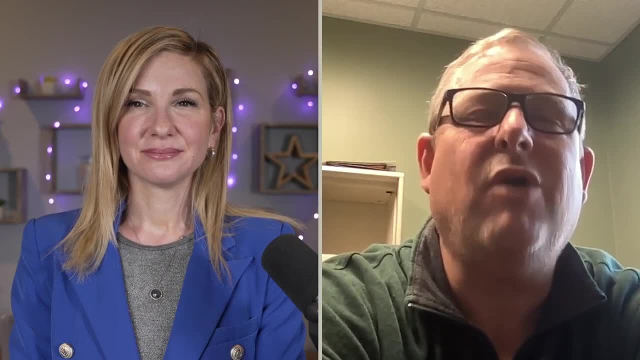 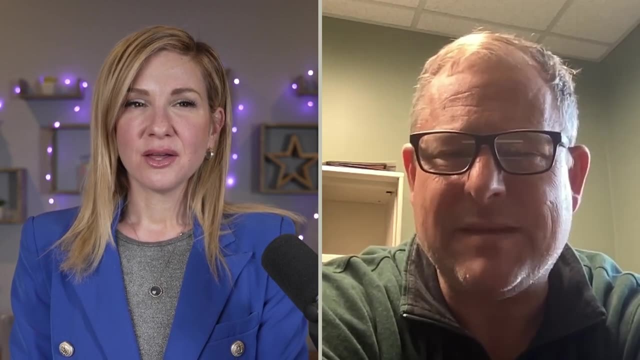 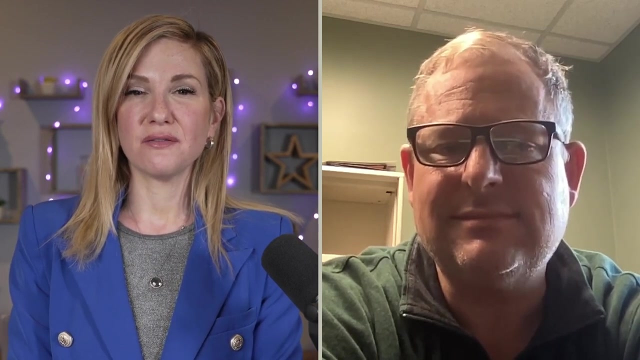 So those are the kinds of sources of unreliability and challenges that we get in the way. this is done by a lot of companies. I'm so glad you said that, Boris, because this idea of reducing back-end complexity of fixing process, that is a huge piece of an improved customer experience. 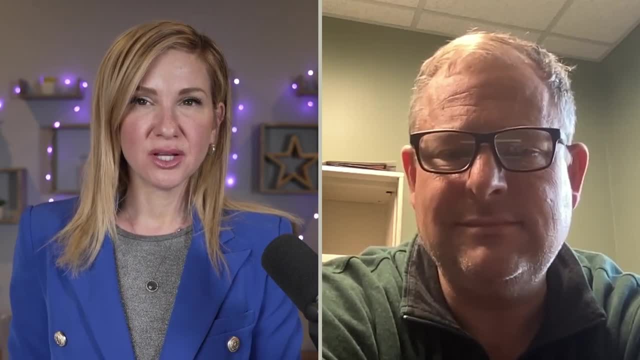 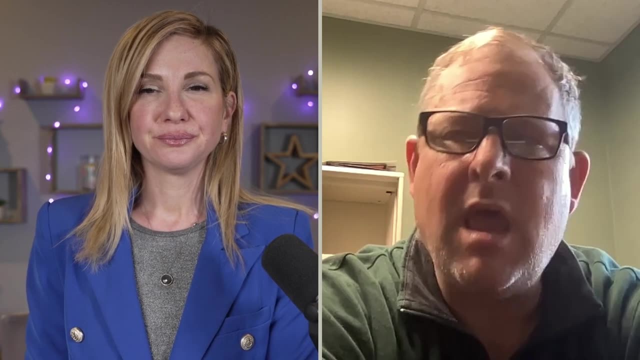 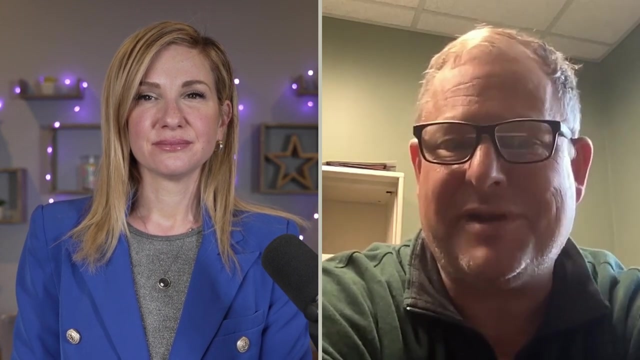 But it's one that we don't really talk about as much as we should. What do you think are the tenets of a really strong? It's a tricky question, in the sense that I would really want to define what kind of good we're offering to a consumer before I answer that question. 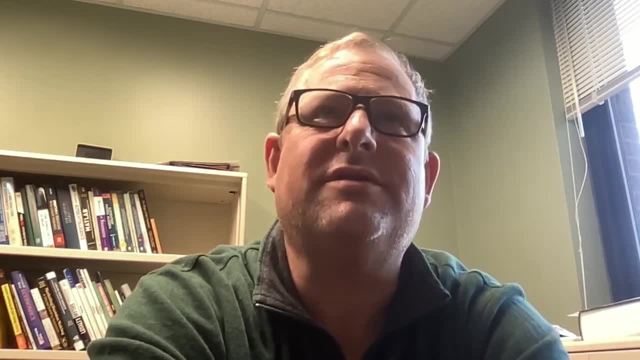 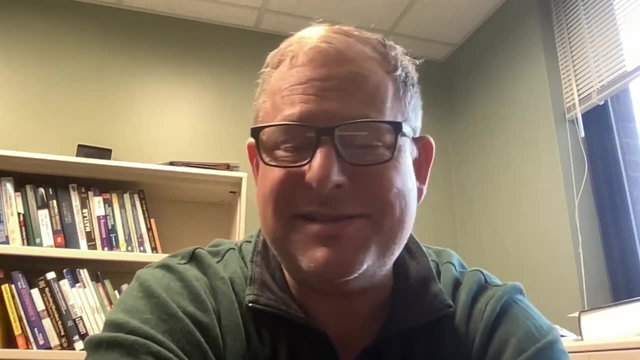 But I mean there are certain tenets, I think, getting to your question, There are certain tenets that I think apply across virtually every industry, And you just touched upon one a moment ago. I mean ease, How easy is it for me to do business with you as a company? 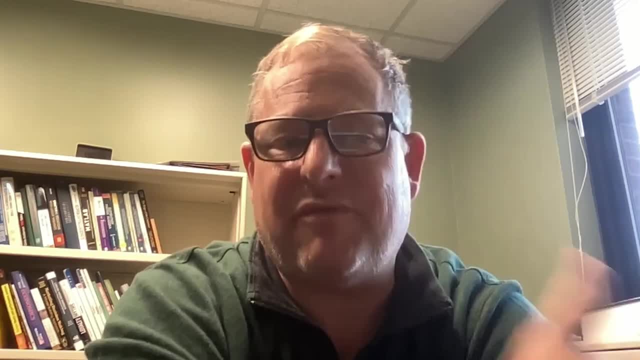 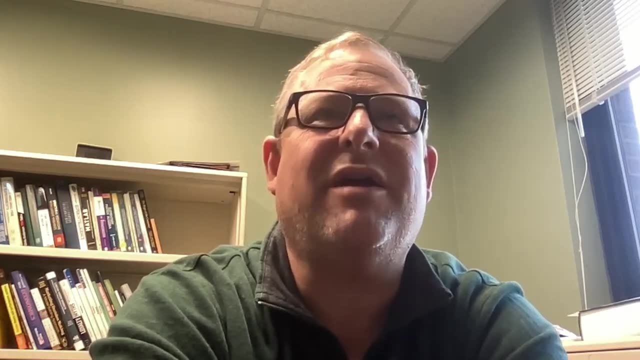 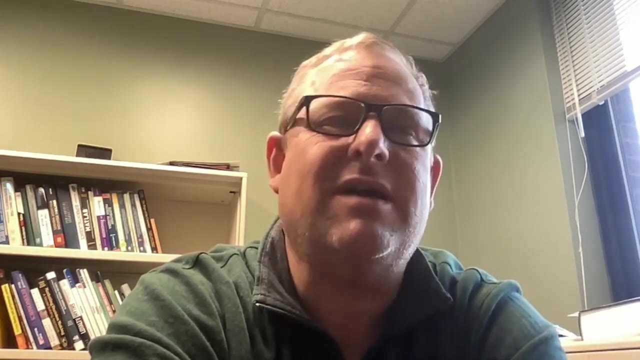 Do you make it challenging for me to become a customer, For me to stay a customer? That's always a bad idea If it can be avoided. if you're in a regulatory environment where you can allow customers more frictionless sorts of experiences, then you definitely should do so. 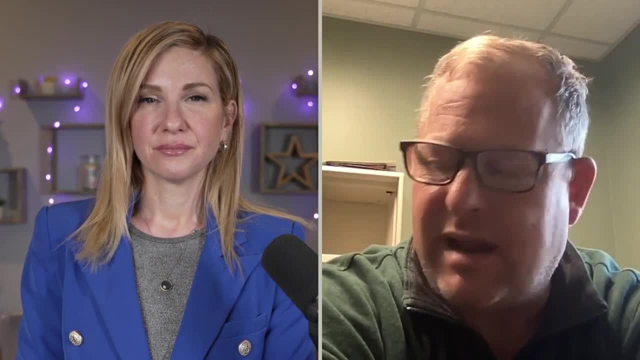 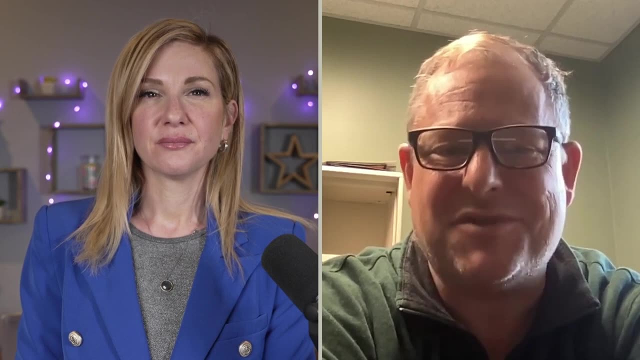 Do you have customer service? I was reading a great article yesterday about how consumers are really starting to stand up and rise up against self-service checkout technologies, self-service technologies at retail outlets. They just don't like them, You know. They're difficult to use. 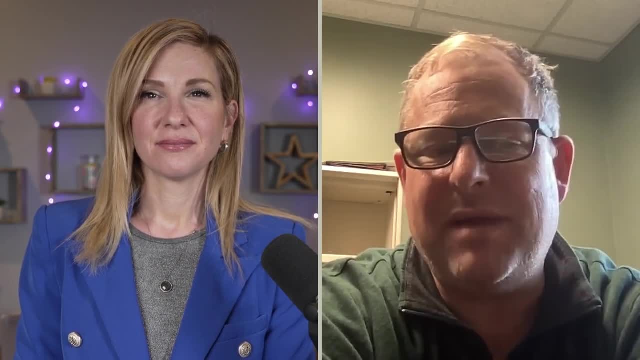 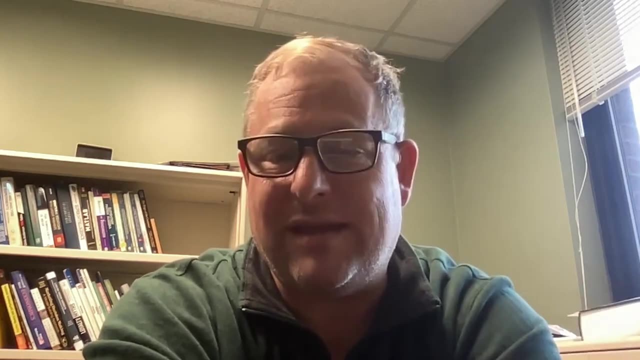 They're time-consuming And the retailers are starting to admit that there's greater loss from those technologies than once was believed And it may not be worth it, At least until those technologies get better. maybe it's just better having human beings doing the checkout process. 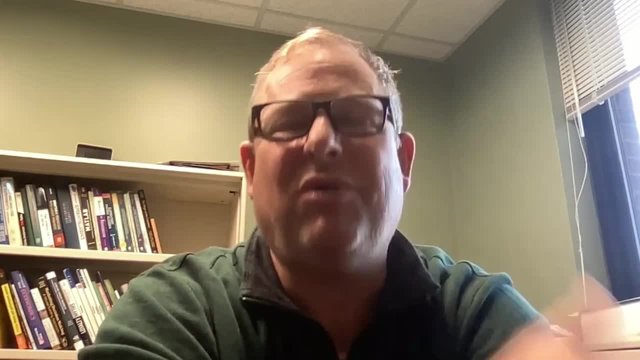 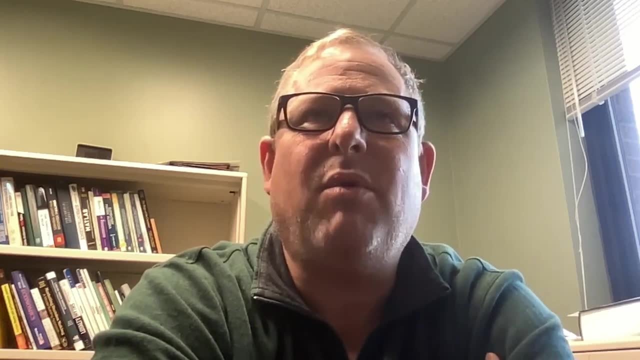 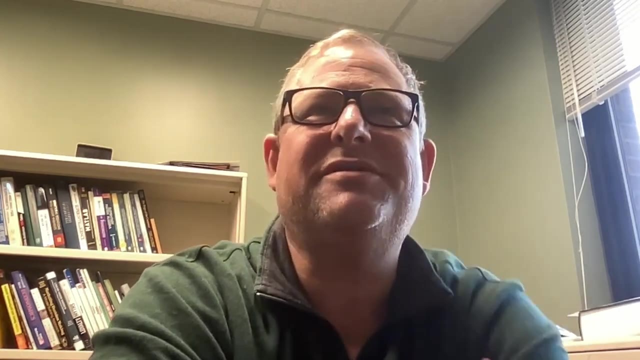 You know how easy is that checkout. How can we deploy those technologies in a way that customers like? And that sort of dovetails into another point: Is the customer service delivered by humans? Is it delivered in such a way that consumers feel a relationship with brands? 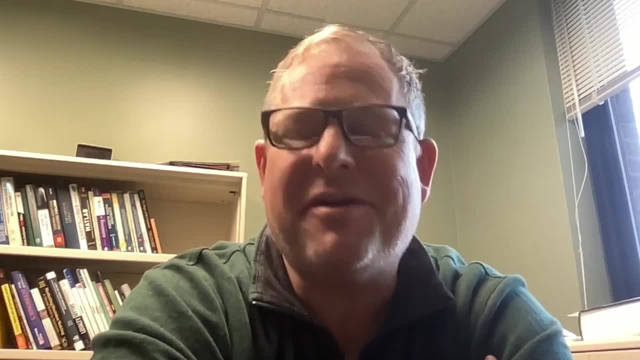 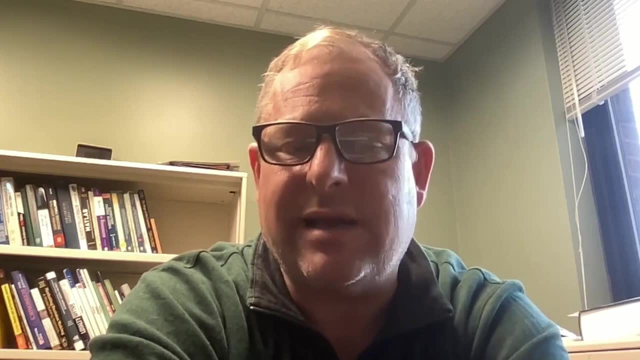 Where that's important. It may not be important in every industry or context, but who am I getting my customer service from And how is that impacting the way I feel about the retailer or other business? Yeah, absolutely, I love the checkout discussion. 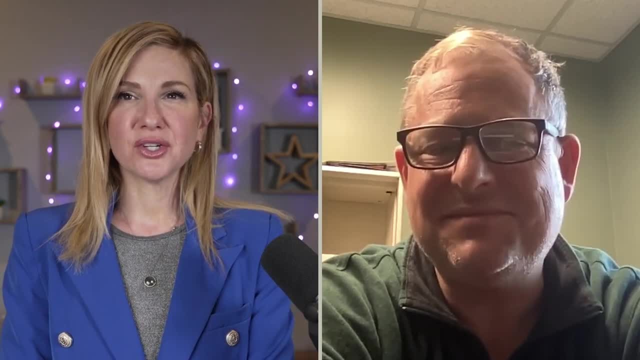 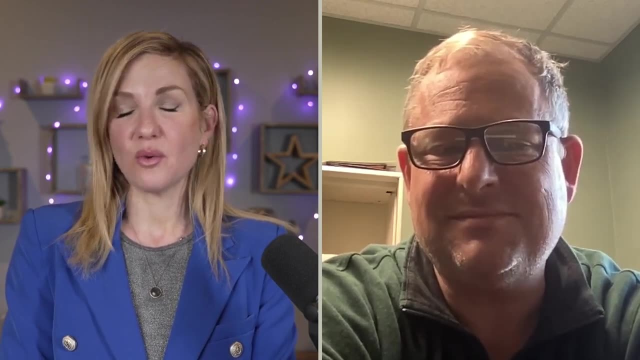 It reminds me of Trader Joe's. I was just thinking about this earlier how at Trader Joe's they don't have self-checkout, And part of the experience is when you walk up to the register and a friendly employee in a Hawaiian shirt asks you how your day is going. 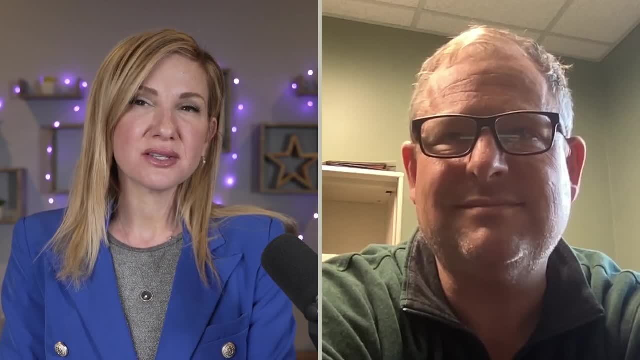 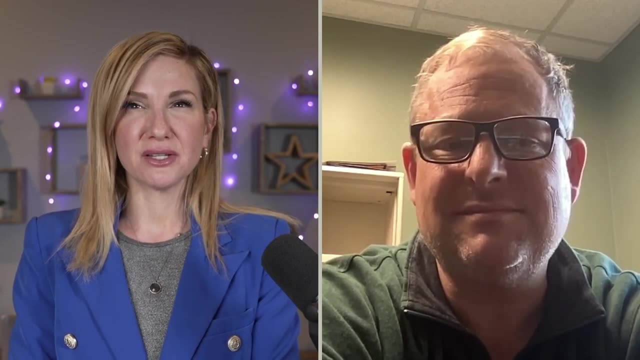 They'll comment on the food that you bought. Oh, you know this is a great recipe if you use these almonds in this way, And it really enriches the experience. So Trader Joe's is like a good mood shopping experience, Sure. 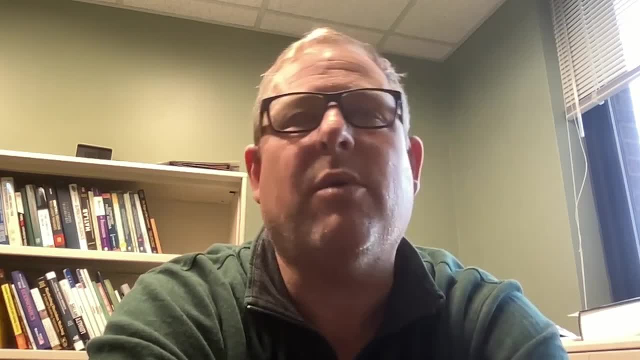 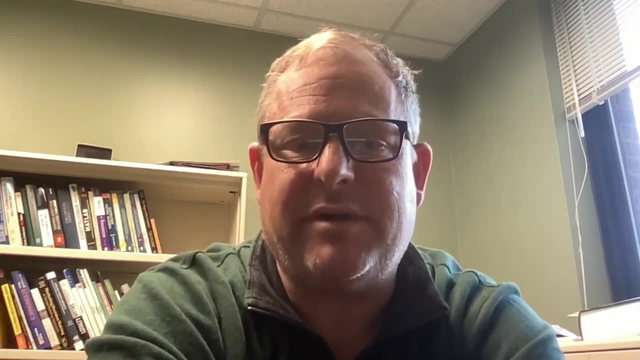 I mean, it's a personal touch And in the era that we're in, where self-service technologies have become so predominant, it's a differential And I think that's a great indicator for someone like Trader Joe's to still have human beings and that ability to make a human connection. 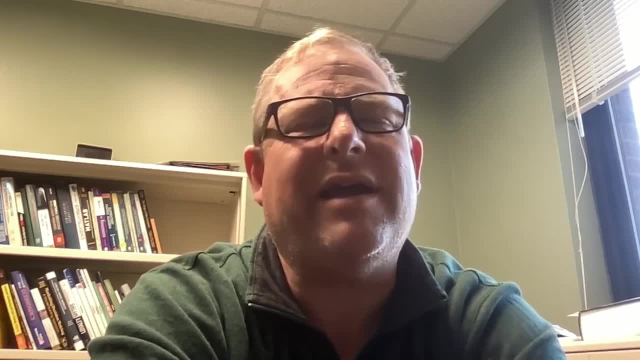 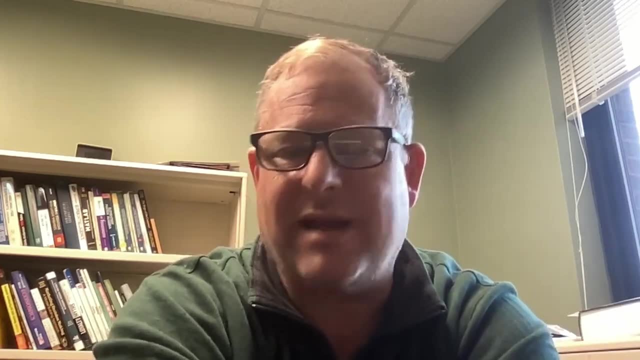 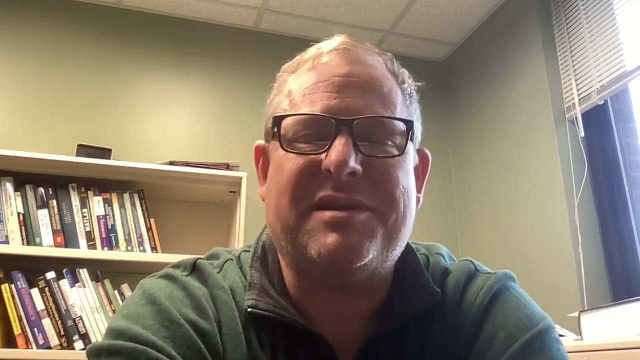 And you've seen, there's a supermarket somewhere in Scandinavia- I can't remember which country- that's now encouraging their people to talk to the customers at checkout as much as they want To make it a friendly experience, To make it an experience rather than a transaction where they're trying to rush you out of the store as much as possible. 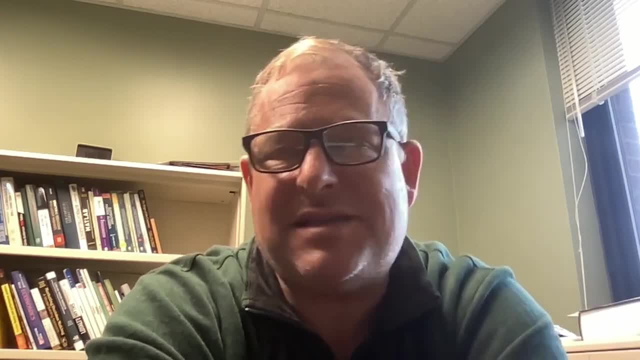 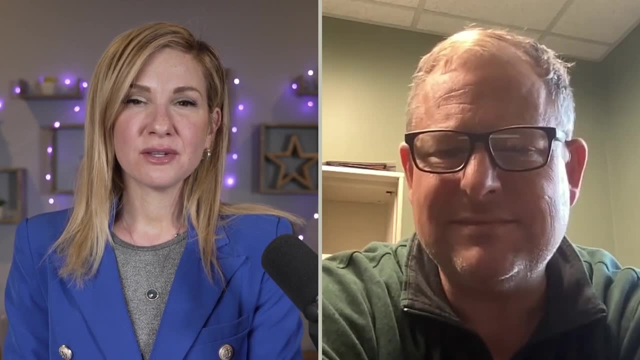 And you know to have that human connection And so that's interesting And I think that's going to become sort of a differentiator for some retailers. So you're a professor And one of the things about being a professor is you do a lot of storytelling. 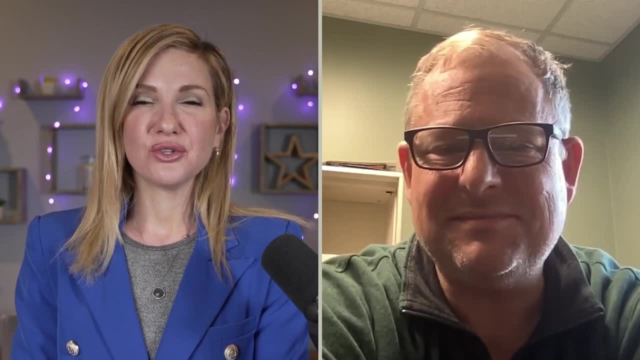 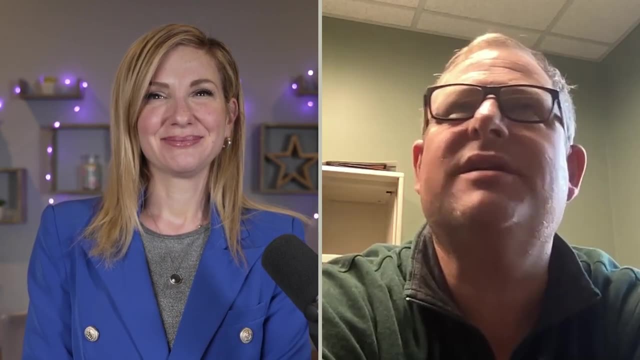 So are there any stories or examples that you tell your students that you really like to talk about, Any case studies you could share with us about good customer experiences? Good customer experiences Or, just as a customer, what you like, Right Yeah. 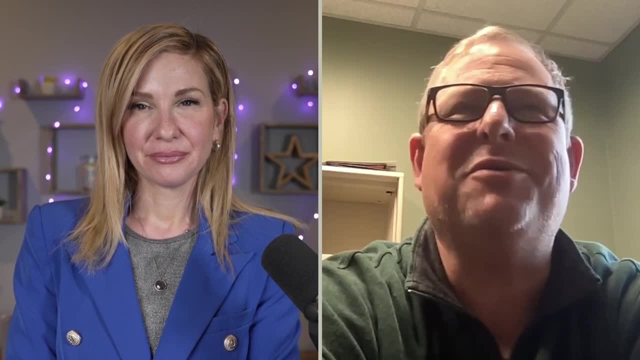 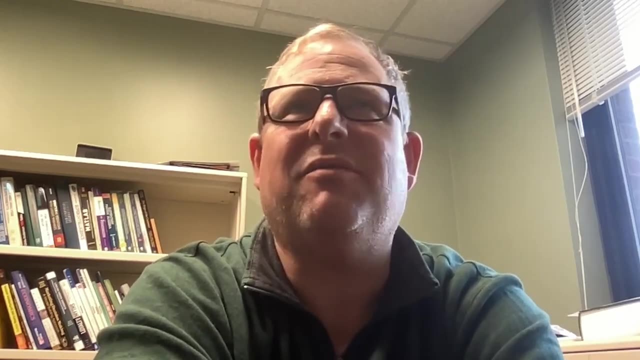 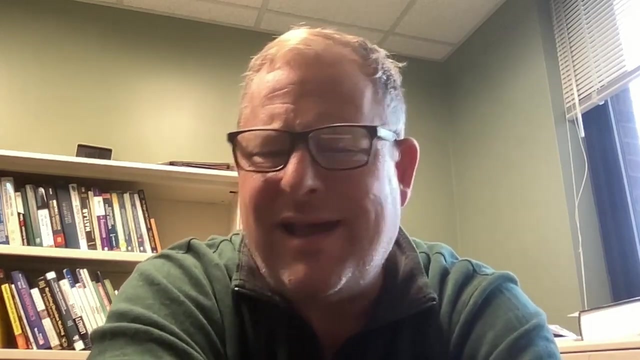 I mean, you know I'll have anecdotes that I will occasionally talk about along these lines. You know, There's the when, above and beyond The company that really exceeded expectations in some meaningful way. And there's, you know, several stories about Costco and managers replacing products for customers by personal delivery after they've had some kind of defect. 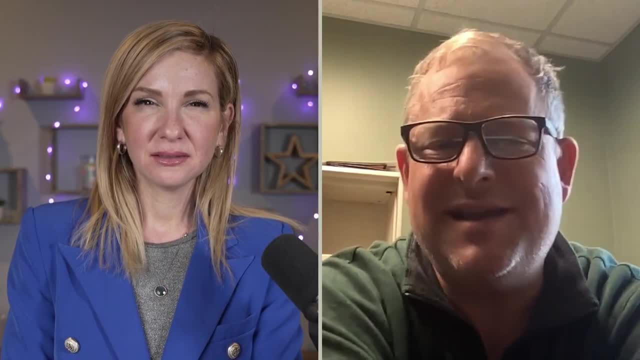 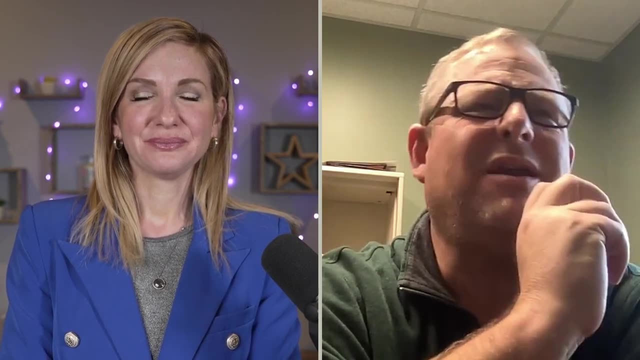 And you'll hear those kinds of stories. What was the company? Costco? This was a Costco story. I can't remember the precise details, But you know it involves a manager, you know, finding out that this customer's product failed. 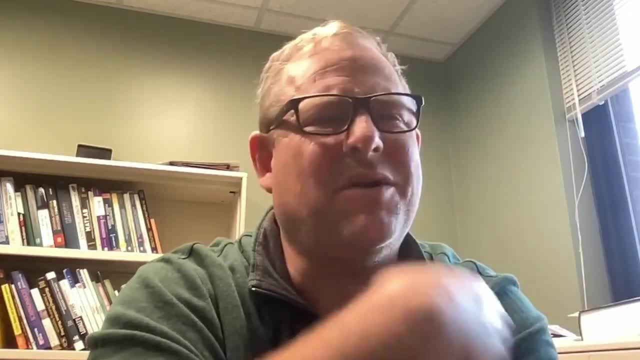 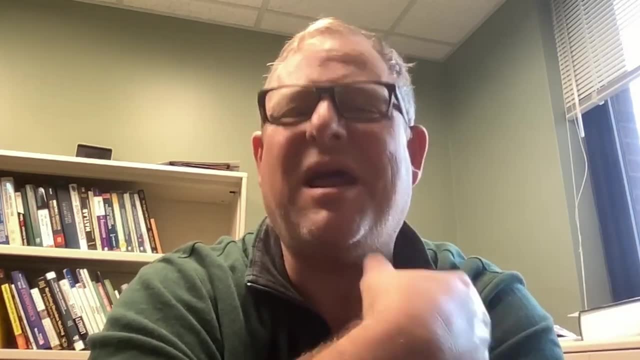 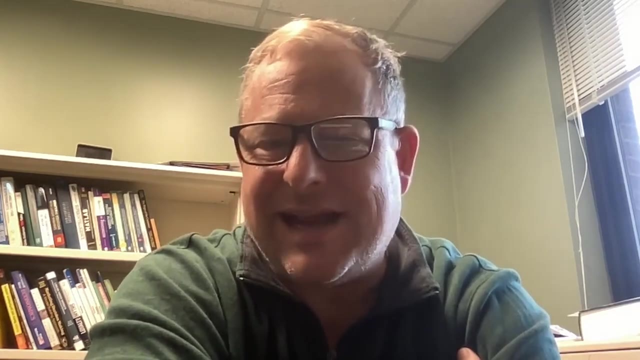 And then personal Delivering the product to the customer- long-running customer. You know those kinds of stories are always inspirational, But of course they're exceptional, Right, They don't happen often And I think you know for most businesses the idea is not to try to, you know, go crazy like that and exceed expectations. 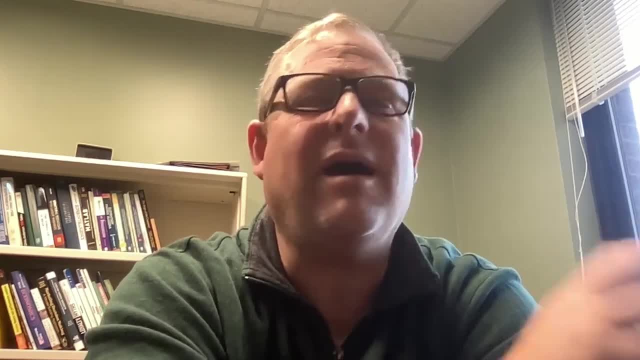 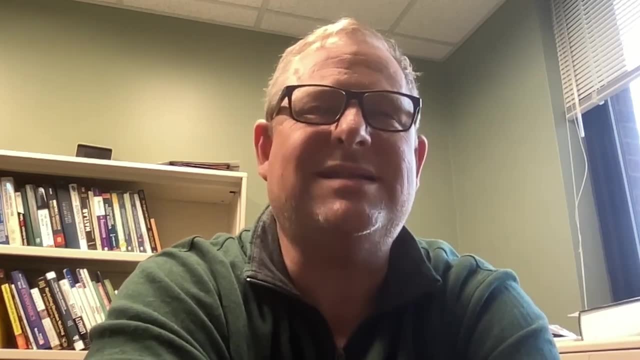 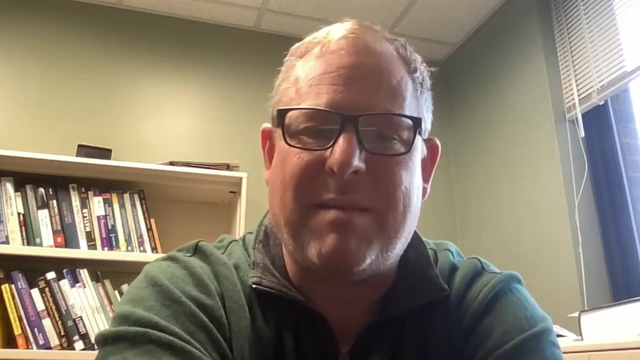 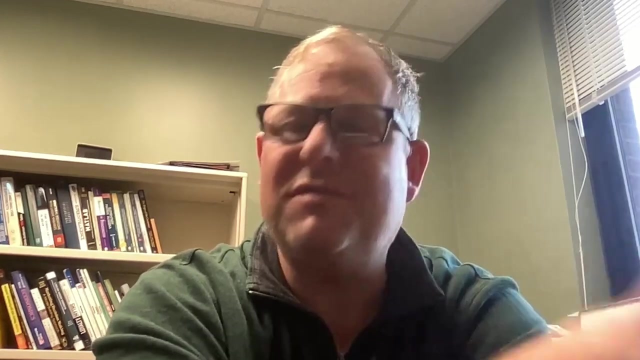 If you have a manager that can do that and win a customer for life through those kinds of exceptional experiences, that's great. What we want to do most of the time with businesses is not focus on being Outrageously exceptional, but rather being highly consistent and fulfilling our promises, meeting those expectations every single time as being a much more achievable goal and one that will sort of reap rewards over the long time. 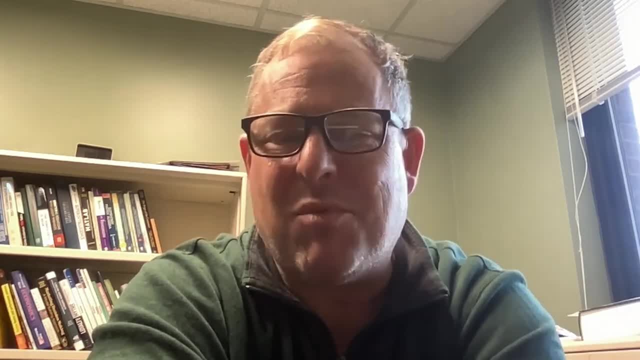 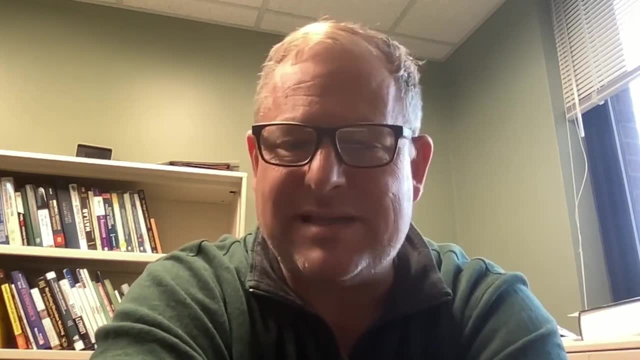 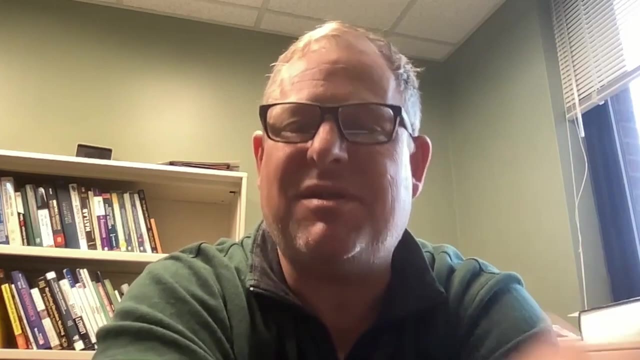 So, in terms of storytelling, I try to tell that more- maybe a bit boring story right- That our goal as businesses is not to overwhelm individual customers with amazing experiences, but rather to provide the whole of our customer base Slightly Better than average experiences, something that they'll get. that's consistent every single time. 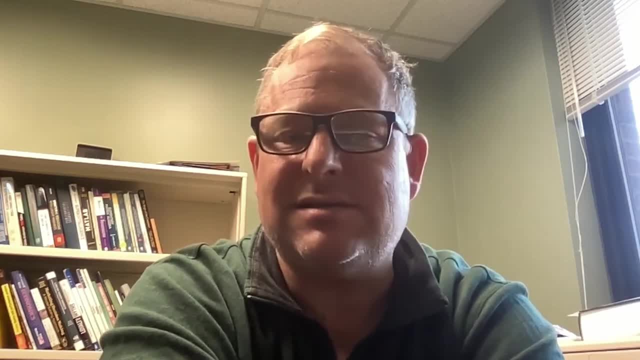 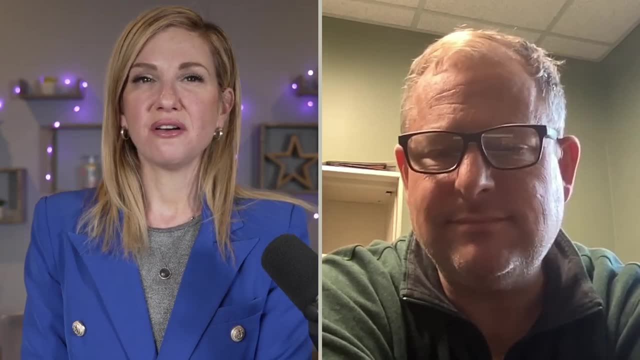 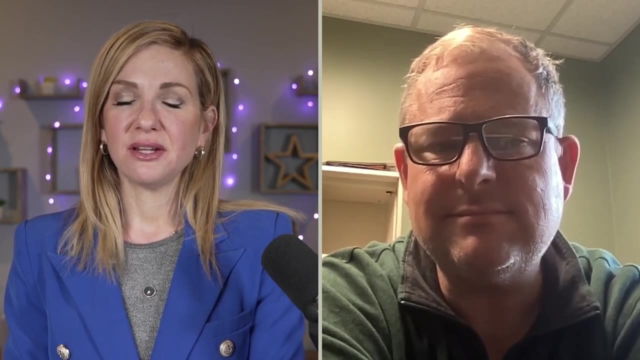 And for that reason it's exceptional. It's it never fails, to the extent that that's possible. So I know that on the research team you are in charge of advanced statistical modeling and analysis. you know, for customer data This is a complicated issue and it's sort of a math of customer service, if you will. 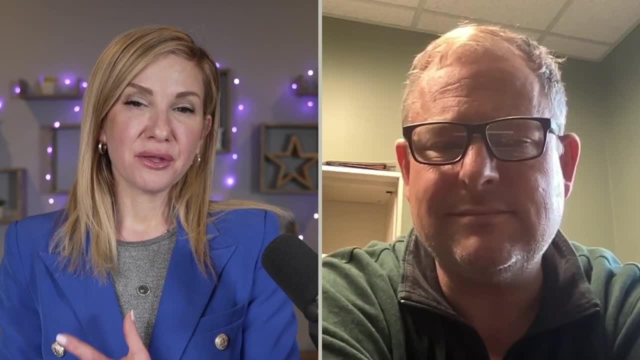 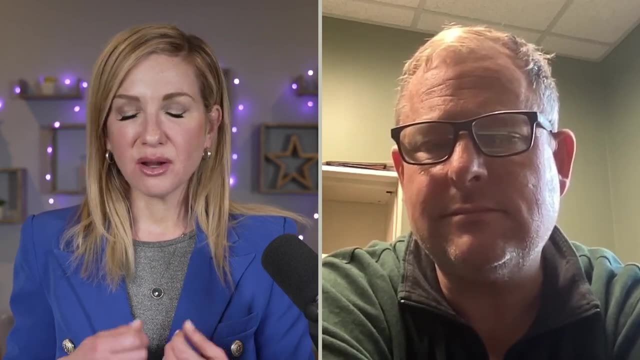 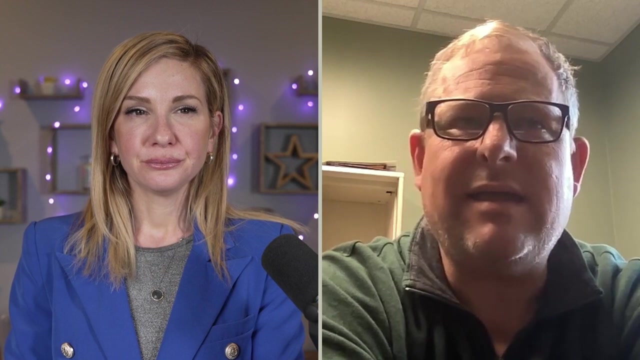 Do you have any thoughts about Literally the math of customer service and how you know we generally measure and manage and what numbers we're looking at, and if you think that's about to change? I mean at the CSI, the way in which we do it is, as you noted, you know, relatively complex predictive analytics. 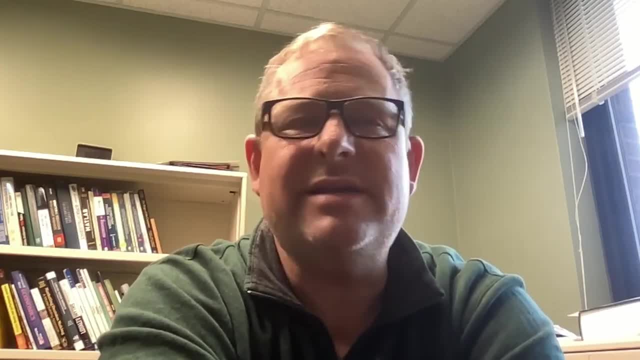 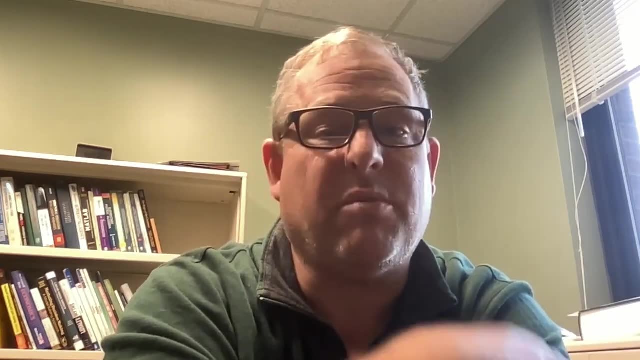 So what we're trying to do is build together a series of concepts and constructs that define the customer journey. if you will, Beginning with you, know What are the things that we're trying to do. What are the things that we're trying to do? 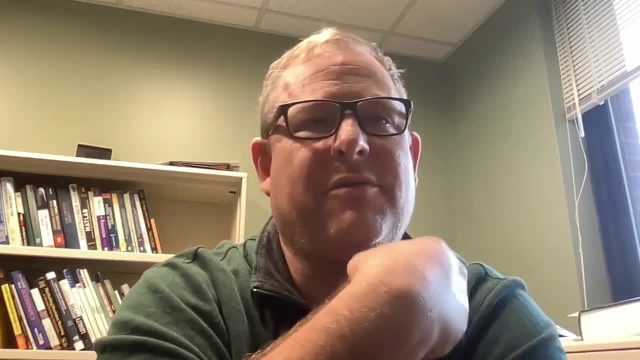 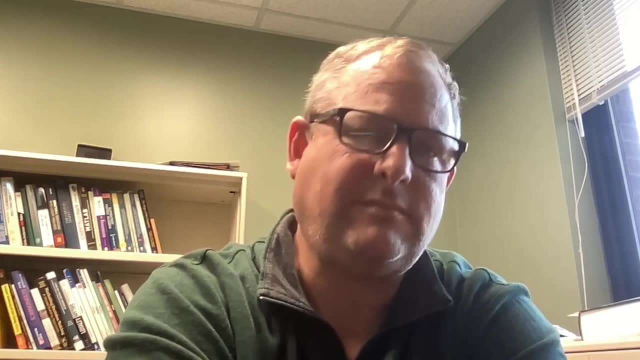 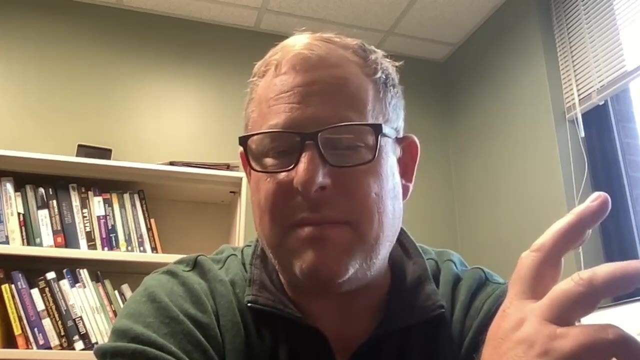 What are the expectations of what they thought they'd get from a business through their perceptions of the performance of that business, How that performance or quality drives their satisfaction? And then downstream consequences of that customer satisfaction, including their tendency to complain about their experience, to negative word of mouth or negative voice. customer voice- 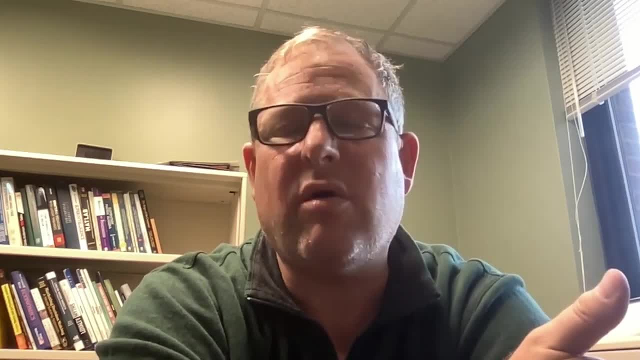 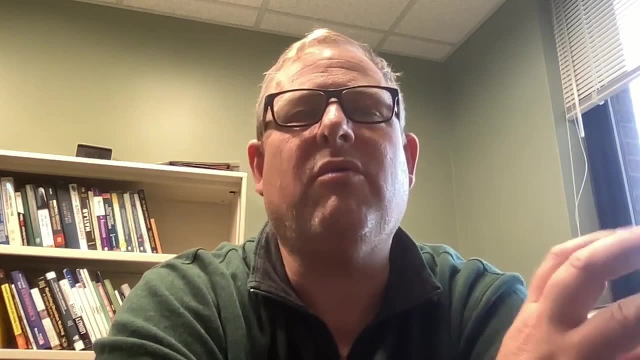 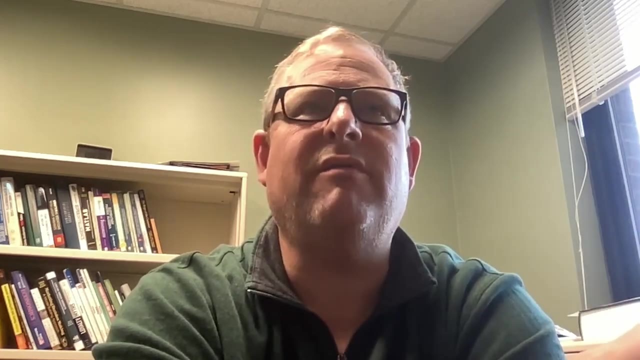 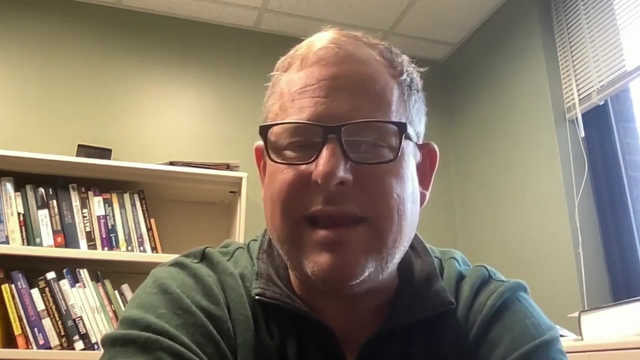 And their likelihood of remaining loyal to a business, paying more for that business's products in the future, Those Kinds of downstream consequences. And so what we're really doing is is thinking about all of those elements of the customer experience as part of a predictive model, where one flows to another, flows to another, and using advanced analytics to quantify those relationships. 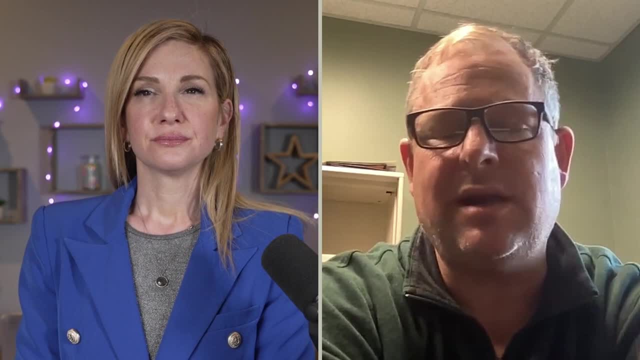 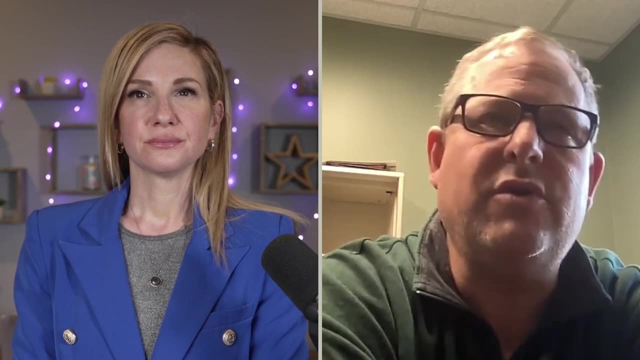 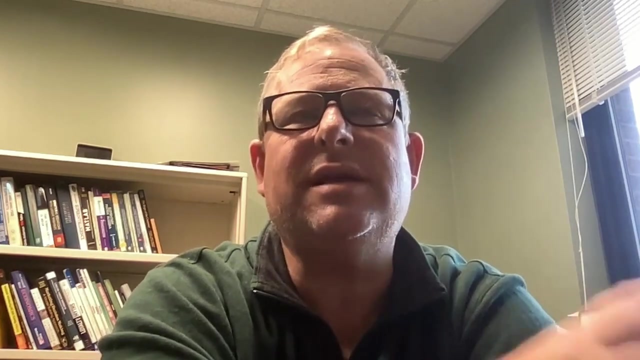 The strength of the relationship between customer satisfaction and complaint likelihood, the strength of the relationship between satisfaction and that tendency to remain Loyal- Loyal in future purchase events to that particular company. You know that it's we've been doing it a long time at ACS using those kinds of methods. 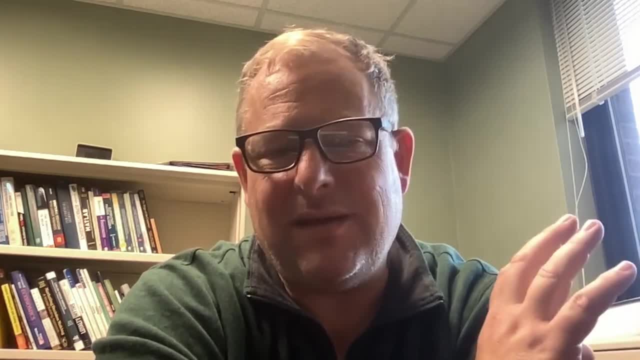 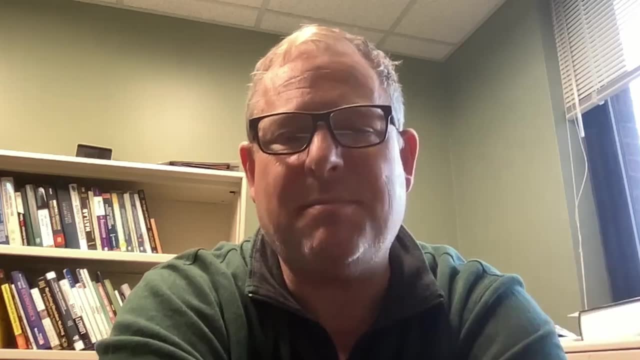 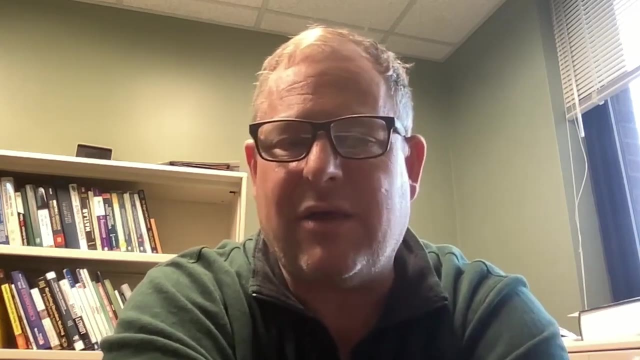 Unfortunately, what we see in a lot of businesses is they still. you know there's complexity in that method of analyzing your customer relationships, And so too many companies rely on much simpler methods, on you know, single items where they measure a you know a single survey question and use that and don't relate it to other important elements within the customer journey. 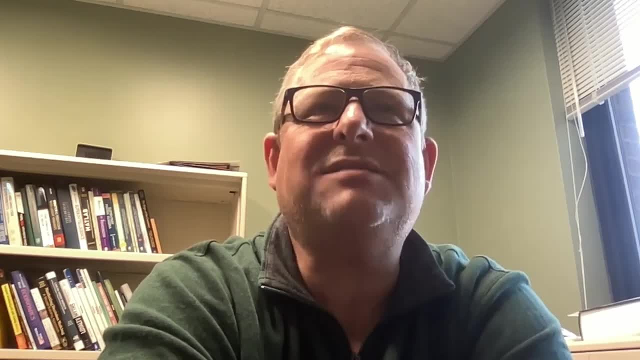 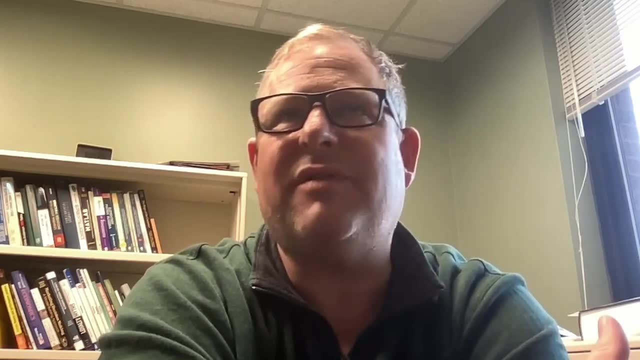 Loyal, Loyal, Loyal, Loyal need. So you know, I think that's my biggest takeaway there. There is complexity to doing it as sort of a predictive model relating a bunch of variables to one another in a robust way. 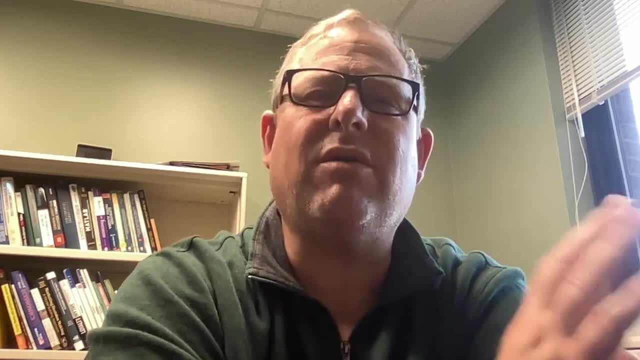 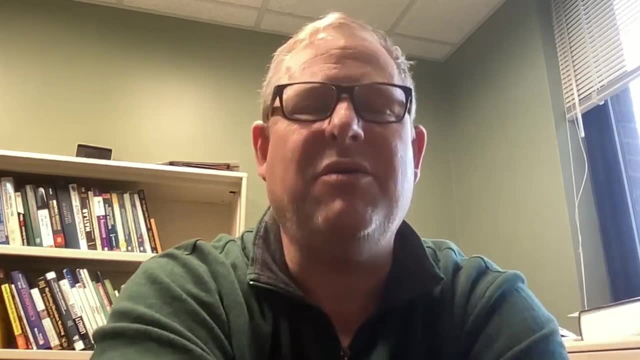 There's complexity there, but it just gives you far better results and a far better understanding of what's really going on with your customers, why they're staying or defecting, and how you can inspire the behaviors that you want to see in the future from those customers. 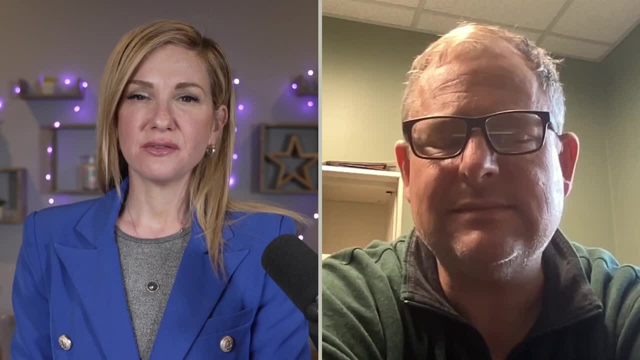 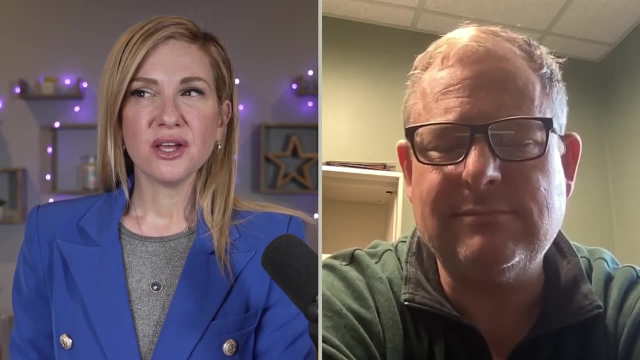 Yeah, it seems like many companies, they're happy to just have one survey question and just keep it really simple so they can check the box. It almost feels like this quantitative data is allowing us to put lipstick on a pig where we don't even see with our eyes anymore what is. 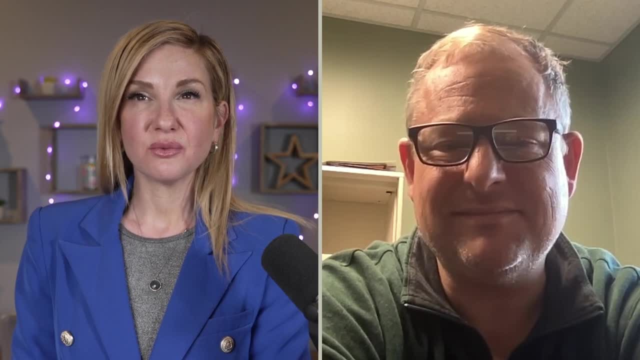 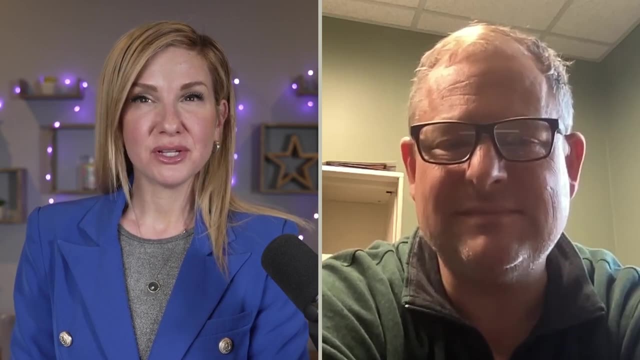 very obvious because we're so obsessed with our data and our stats, We know if our customer experience usually is bad or if it's good. You know, we generally know We can ask our employees. So do you think that there is too much? 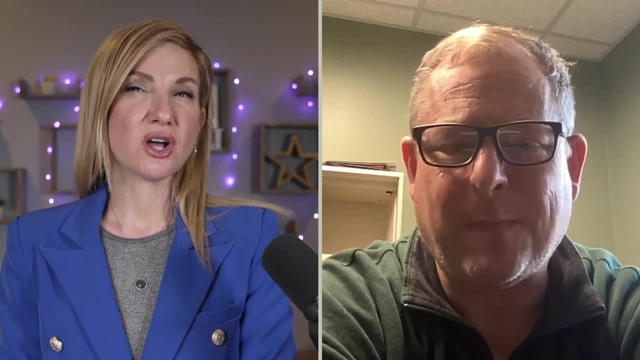 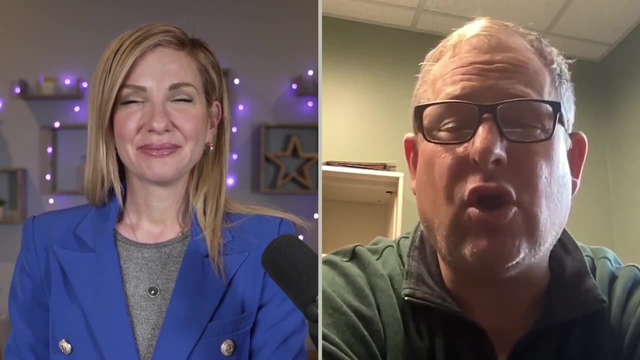 Do you think there's too much focus on quantitative data that you encourage people to talk to customers and look at qualitative data? I think there's many wonderful attributes to qualitative data And I think you can learn a lot about your customers from relying on more qualitative types of methods, observing your 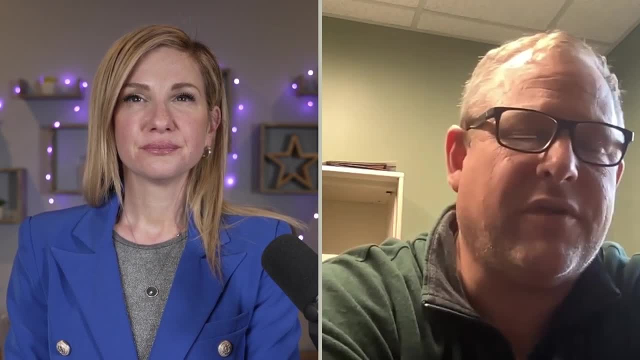 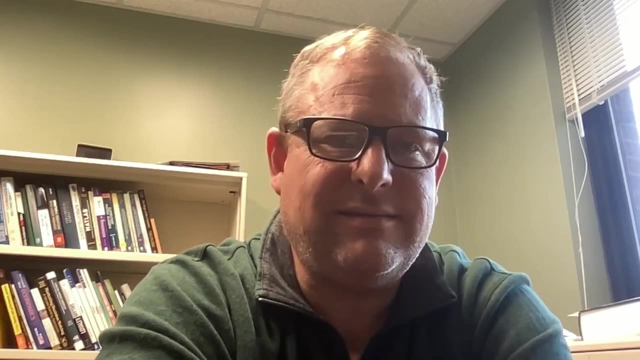 customers see how they're doing when they're wandering through the store. see what they're doing, what they're looking at, what they're not looking at. You know. the reality is that you know once you get to a certain scale it's very difficult to take more qualitative type. 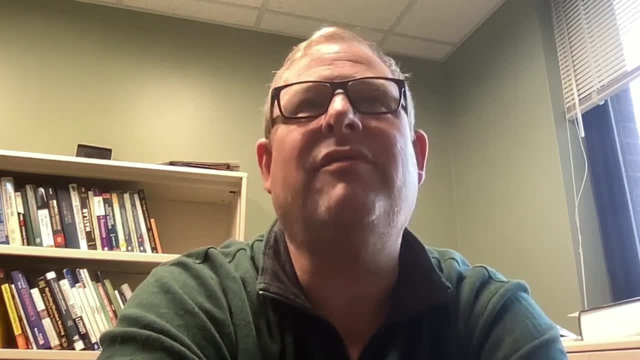 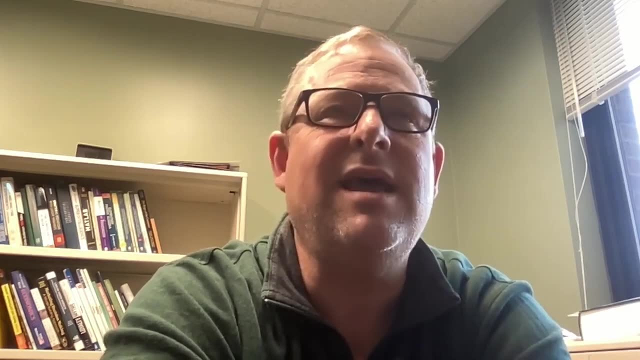 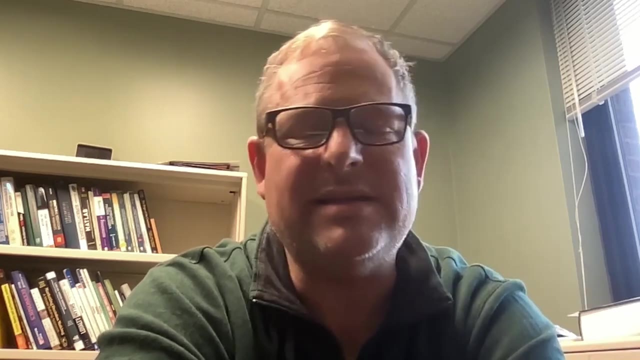 approaches. We need to have some kind of quantitative data, especially if we're talking about tens of thousands or hundreds of thousands or millions of customers of some of these businesses. So I think that's the tendency towards more quantitative approaches in this field in general is, if you're a big enough business, you're going to need to try to quantify these. 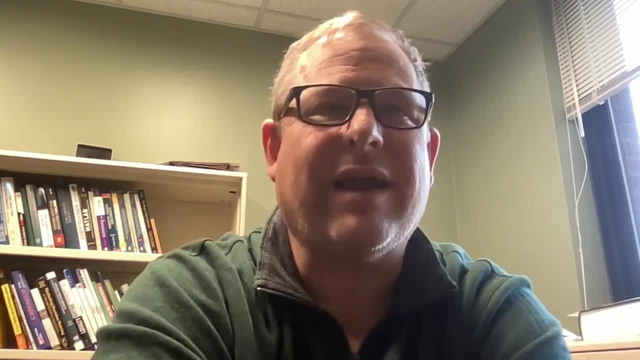 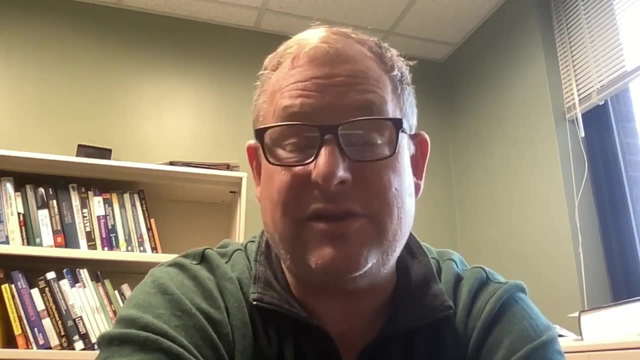 things. Now, what we're doing in a variety of different kinds of market research- and have some of this data at ACSI as well- is taking unstructured data and adding structure to it And turning it into quantitative data, So taking open end responses to survey items. 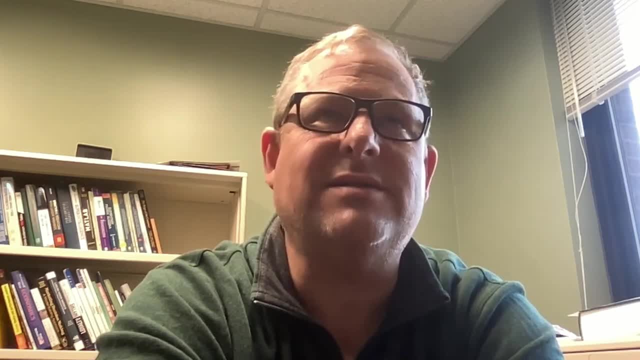 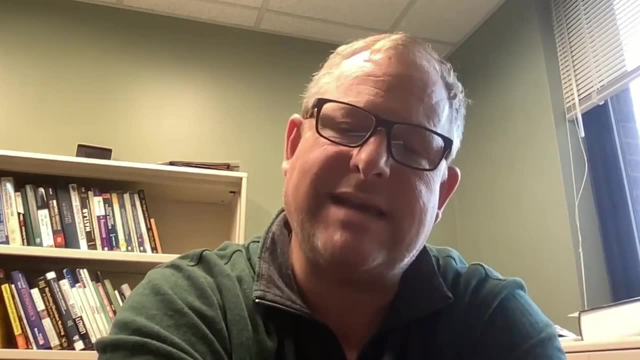 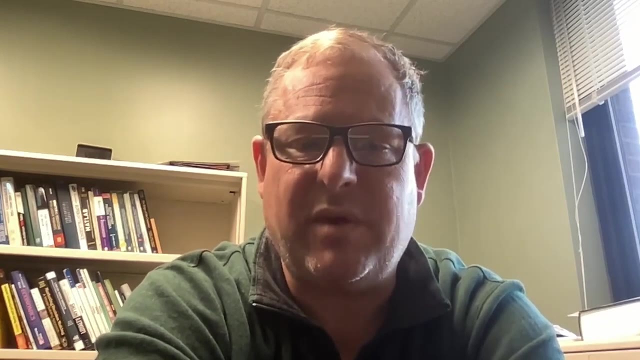 social media comments or comments being made about our brand on social media product and service reviews that you can find through the internet. taking all that more qualitative data and then quantifying it and using it as an input into that model where we're looking at relationships between variables and our customers' behaviors. 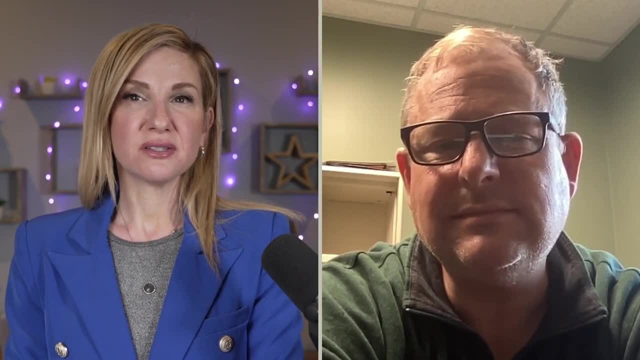 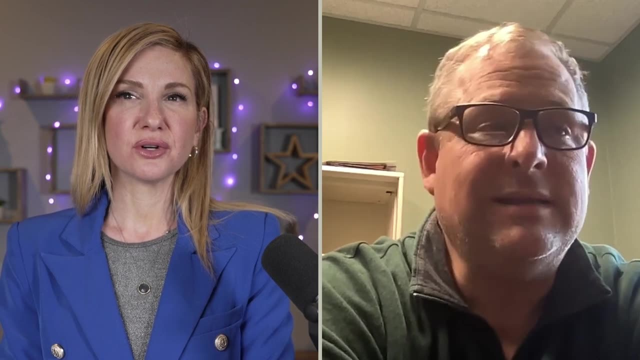 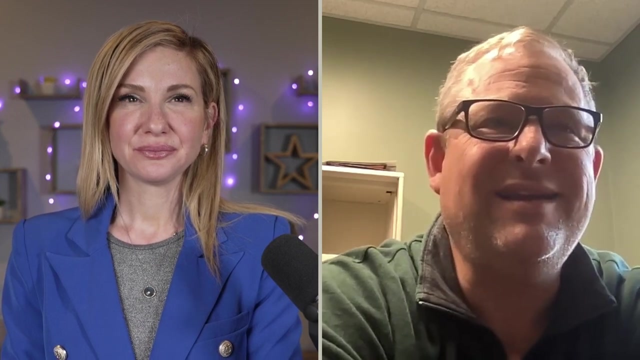 Let me ask you this first: What if you didn't have any surveys At all? There was no such thing as a survey. How would you measure customer satisfaction if you couldn't send digital or paper surveys? Yeah, that's a very difficult question. I mean, it's one of the neater things about this line of 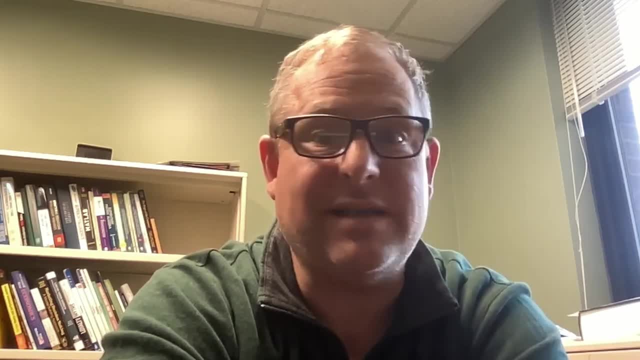 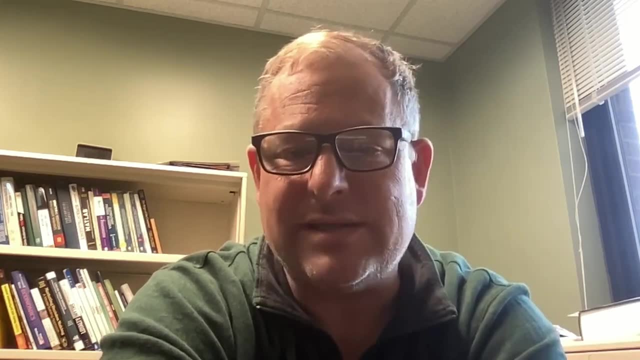 work- or at least us in the business- is that customer satisfaction is one of those things that's not directly observable. You can't directly observe the satisfaction of your customers. You can't even do it with something like customer loyalty. We can count objectively and accurately. how loyal we are to our customers. We can count objectively and accurately how loyal we are to our customers. We can count objectively and accurately how loyal we are to our customers. We can count objectively and accurately how loyal our customers are, Assuming we have their names. 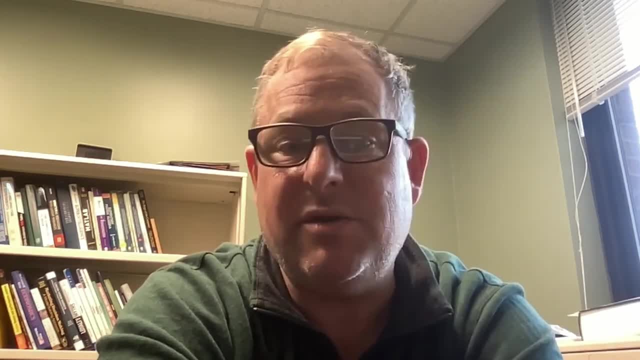 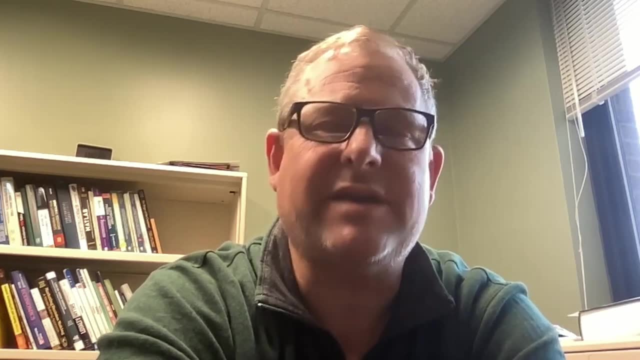 or some other CRM-related database of customers, we can see who comes back and who doesn't come back. But even that isn't necessarily perfectly correlated with satisfaction, because of course customers may come back simply for convenience. They're not particularly happy. 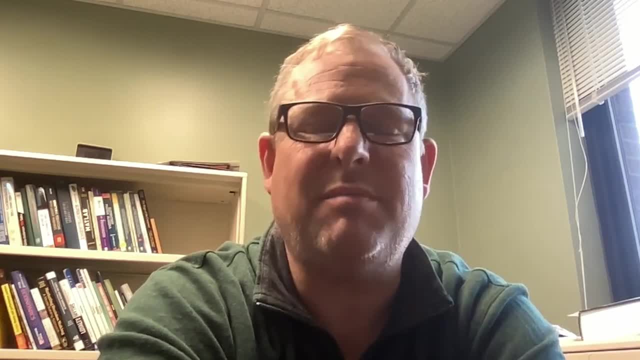 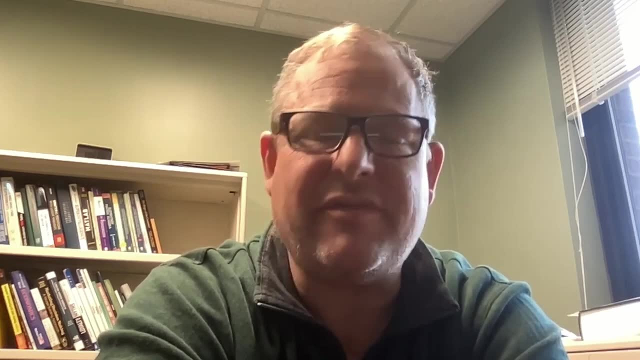 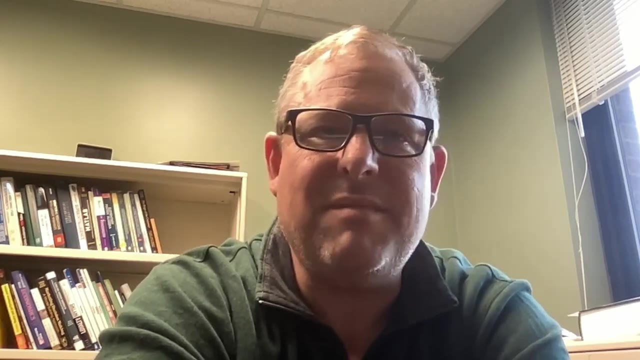 but it's the closest business to them that offers that type of good or service, So we really need to be able to ask about it. Otherwise, we're just trying to defer satisfaction from available data that we think is related to satisfaction. But as of right now, that's still the best way to do. it is to actually ask them. If we can't. 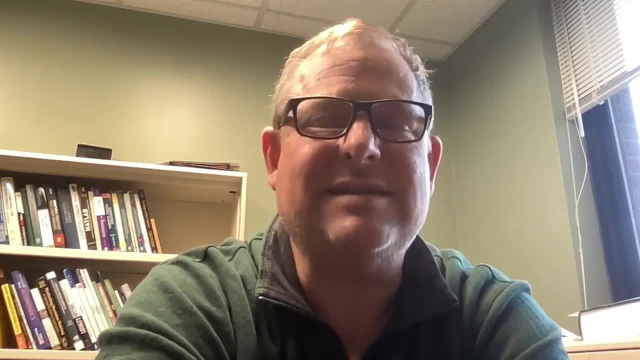 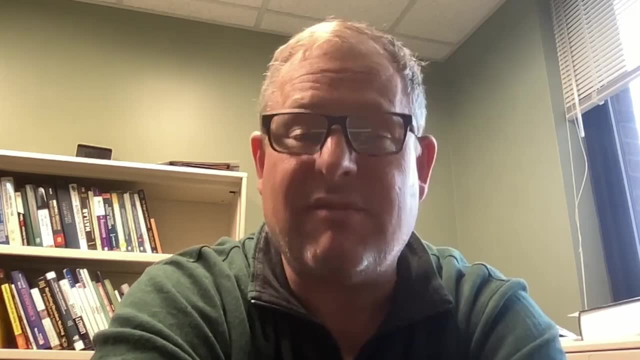 we can come reasonably close by doing the kinds of things I was mentioning: seeing how social media trends are developing when it comes to mentions of our brand, of our products and services. We can look at product reviews, We can do those kinds of things. 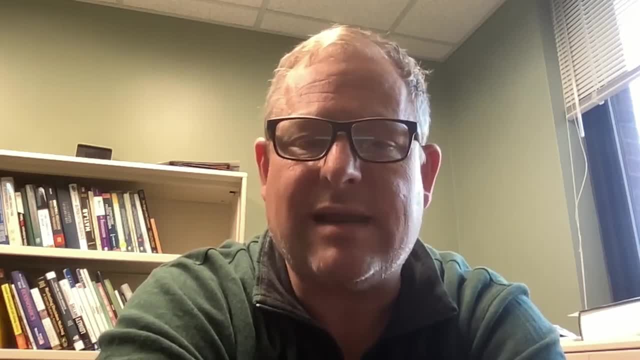 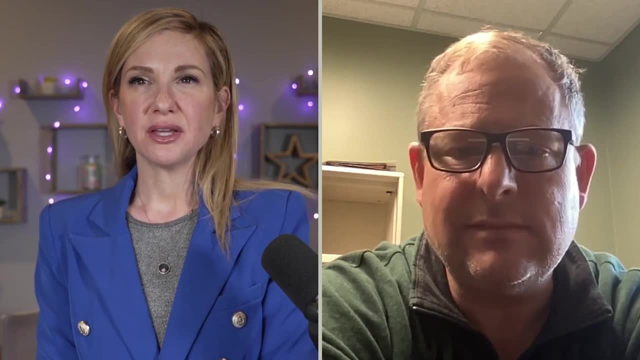 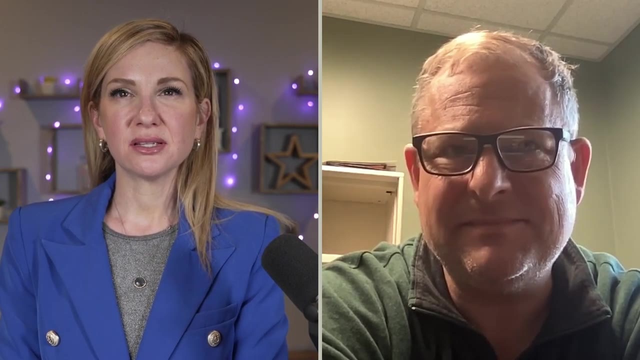 But at best we're getting a proxy of real customer satisfaction. What about earned growth rate, which is Fred Reichelt's new take on net promoter score, where you're tracking how many of your new customers are coming in through current customers? Is that something you guys are exploring at ACSI? 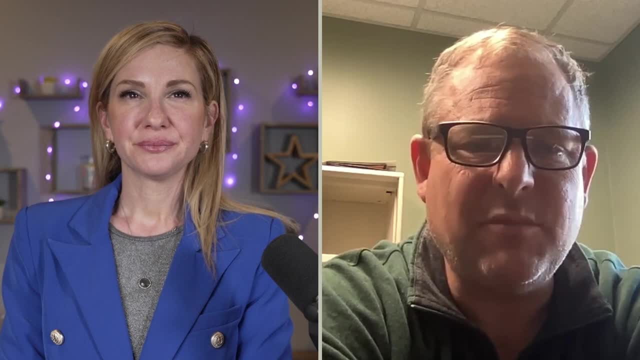 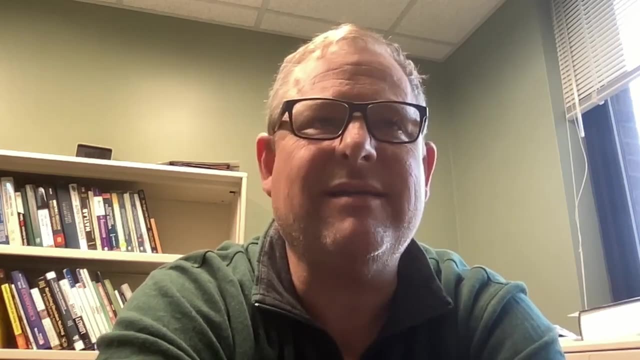 No, not really. I'm actually not familiar with that new concept. Of course we want our products to grow through word of mouth. That's a long-standing thing. Well before NPS, we understood the importance of word of mouth in market research. 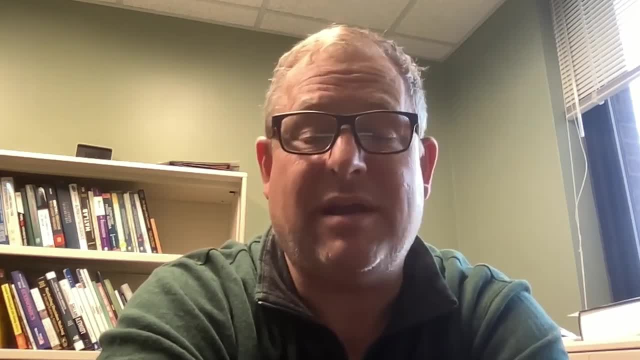 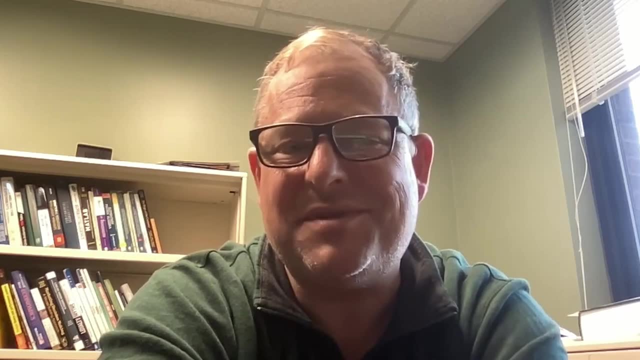 It can be a really valuable source of growth. It can also be a double-edged sword. of course, Word of mouth is not always positive. There is such thing as bad publicity when it comes to your products and services, So word of mouth can be difficult for some companies. But of course, 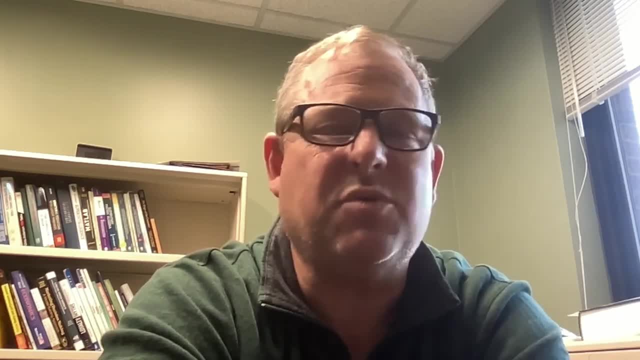 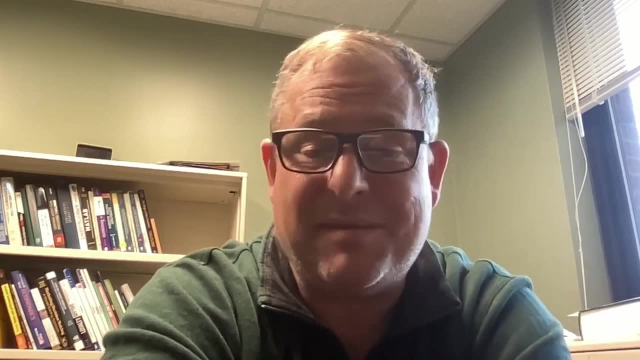 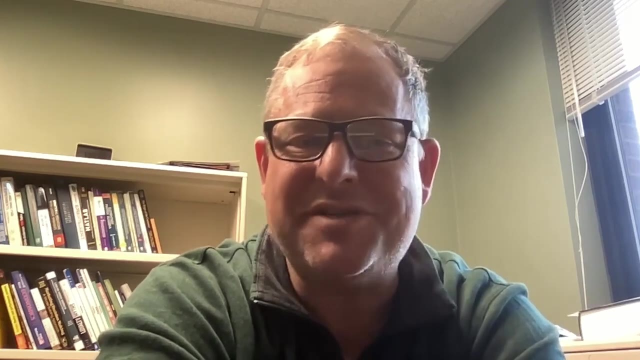 we see a really strong relationship in some ways between word of mouth and customer satisfaction. Dissatisfied customers rarely talk about their product. On the other hand, sometimes very satisfied customers don't talk about their products. The products are too mundane. They don't find them interesting enough to talk about. I don't know. 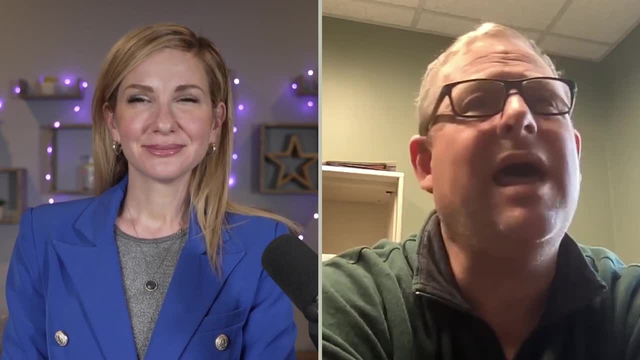 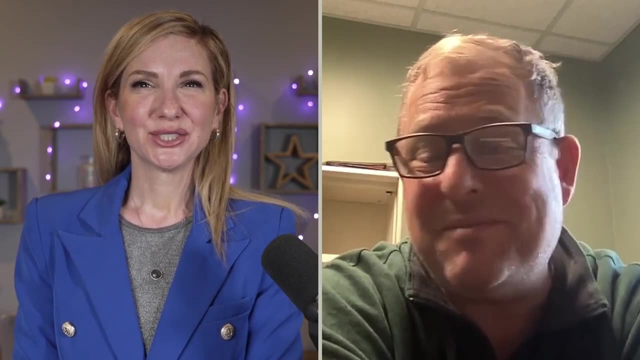 about you, but I don't go to my friends or neighbors and say I had the most wonderful lunch meat the other day that I bought from the store. It was just the best lunch meat. You need to buy it? Some people might, but in my experience not many people talk about that. We may talk about. 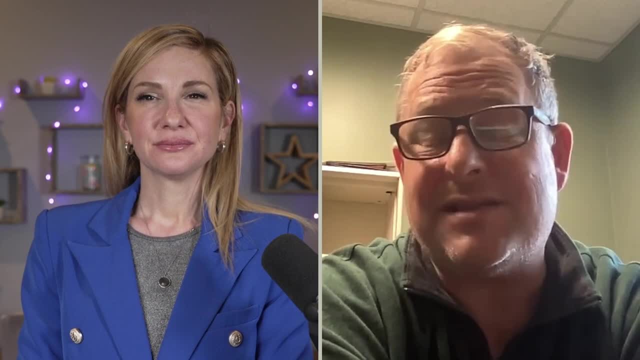 our big ticket items. We purchased a new car and we love it. Hey, I got this new car. I've had it for six months now. You should really look at it. I don't know if you're familiar with that, I don't. 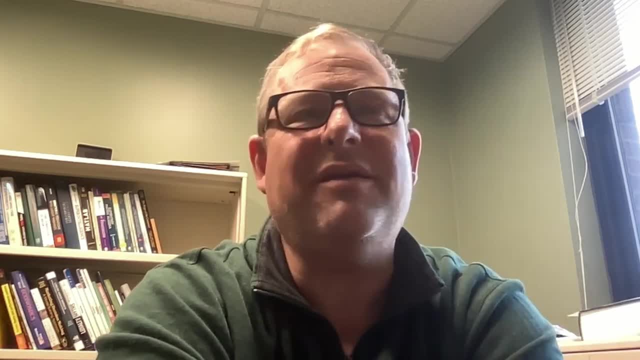 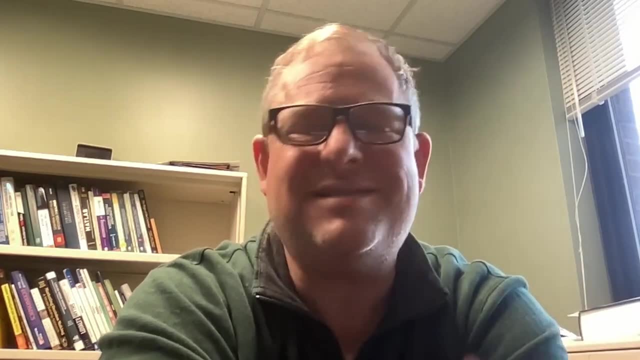 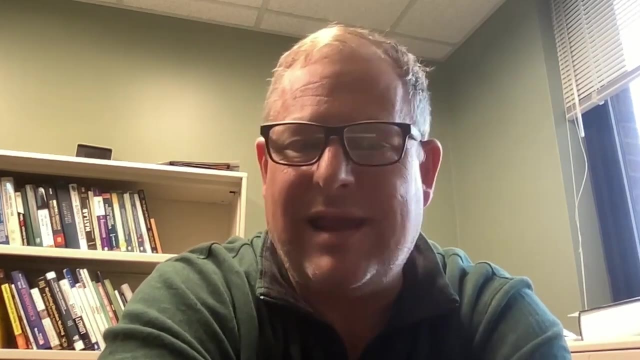 know if you look into it, But there's real category differences there whether or not word of mouth matters. We're really focused on it in the digital economy, because that's what we do in the digital economy. We want to inspire that positive word of mouth and go viral and have our 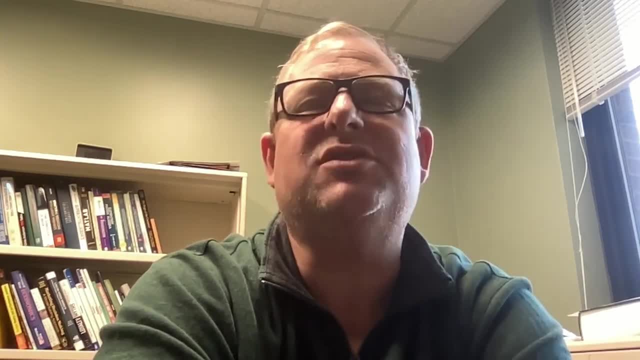 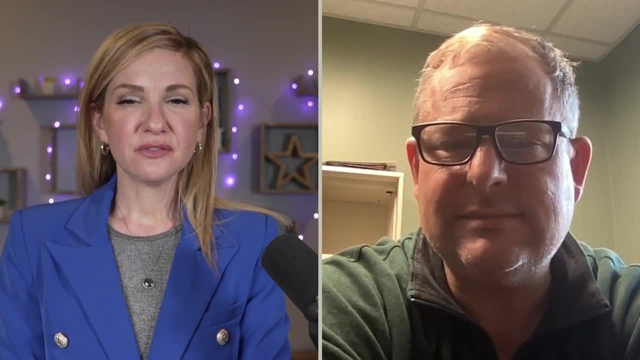 product fly off the shelves. But in reality it's just one among several metrics that we need to look at to understand the customer experience. When I started in customer service, I really didn't want to work in a customer service job. My boss basically told me: oh, you want to launch? 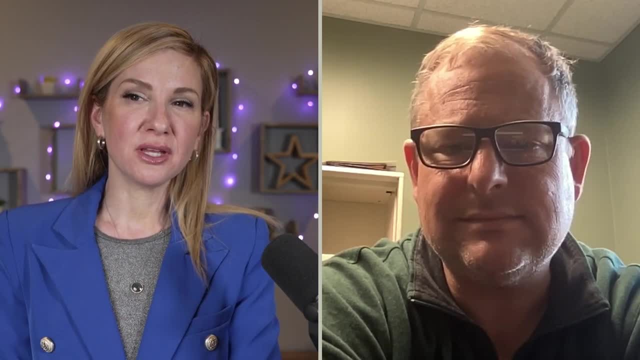 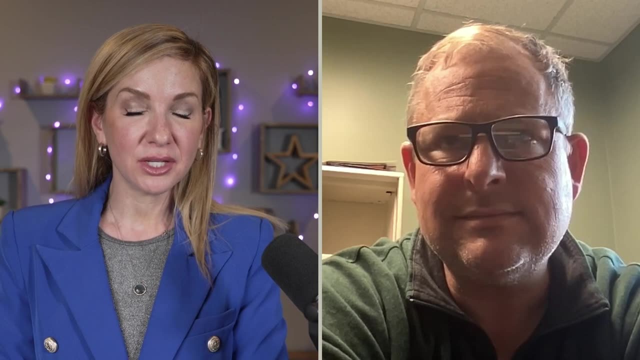 these digital customer service programs. Okay, well, you're going to be the test dummy, You're going to go and try these new channels and you're going to respond to customers yourself, And I really, at the time, didn't want to do it. Now, of course, like many, many years later, I'm very happy. 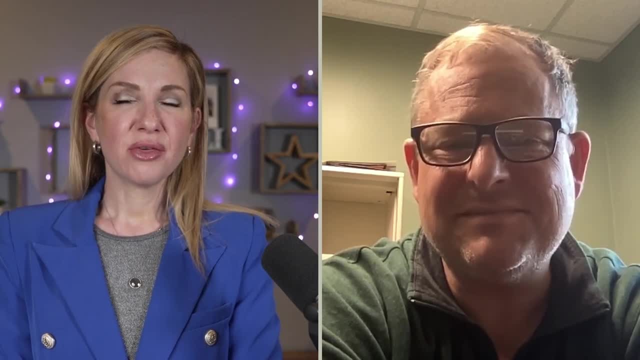 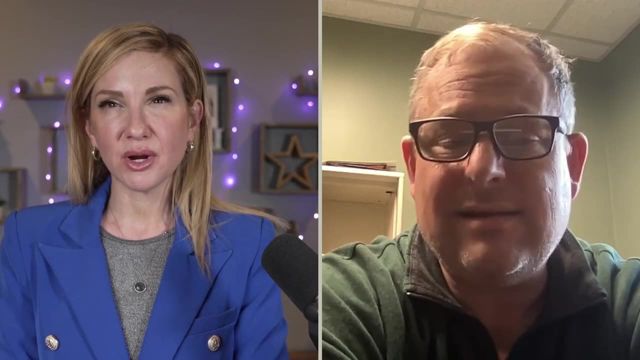 I did. What would you say to a young person that thinks customer service is boring and isn't an interesting business pursuit? Would you tell them that it isn't a good thing? Would you tell them boring? Well, a lot of my students, in fact I got done teaching about an hour ago- are studying. 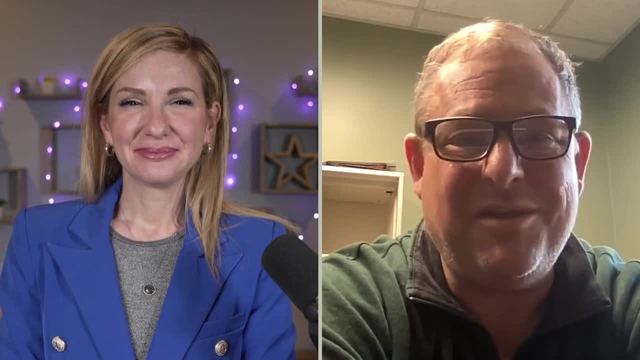 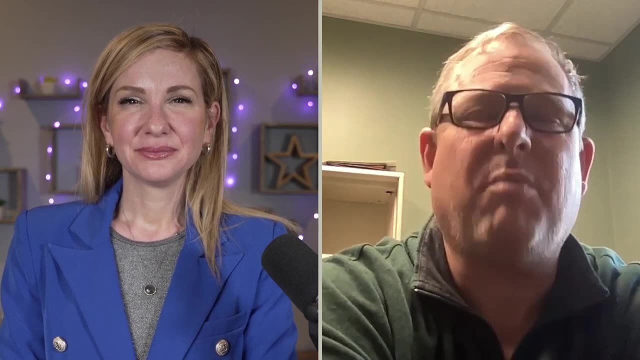 to be marketing researchers, And one of the things I tell them is that, hey, you've got to get there on the ground if you want to understand this. And this doesn't just apply to master's students, who are more practically focused on going into careers in marketing research, but PhD students as well. 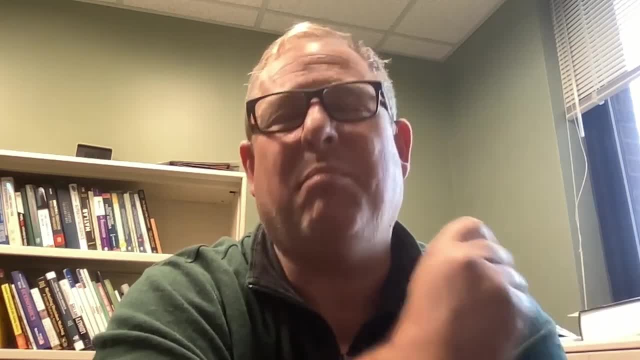 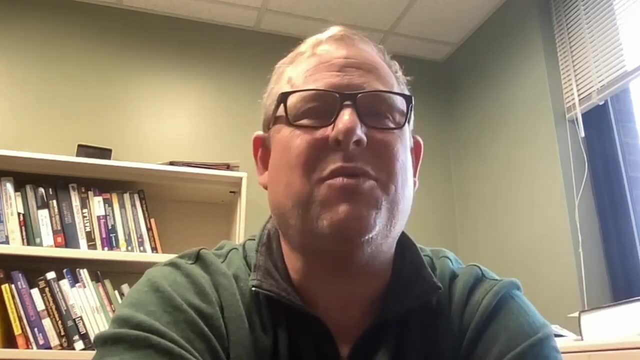 If you want to understand marketing and understand this stuff and ask important questions that businesses are going to be sort of struggling with and trying to address, then you've got to give them answers to those questions in a way that's helpful to businesses. You need to. 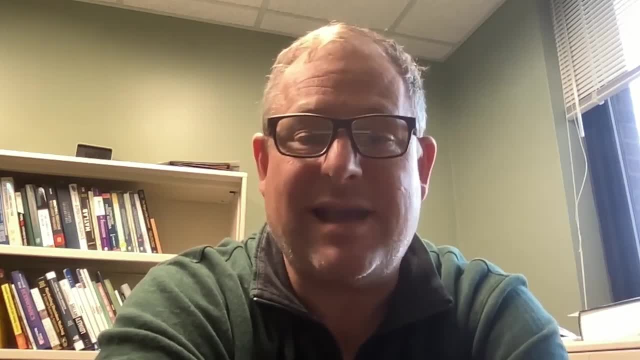 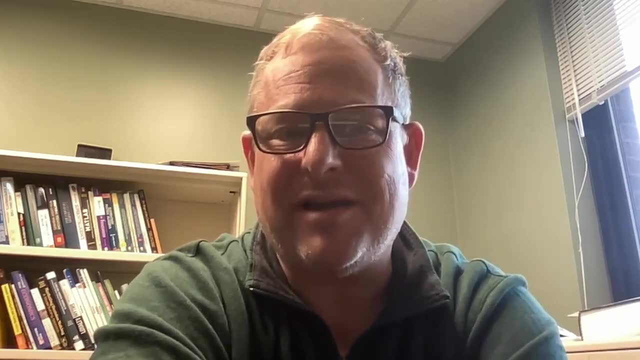 understand what it's like there on the front lines, at least to some extent- And part of that is working in customer service at some point and at the very least, observing what it's like for customers to go through those experiences and maybe better in some way better understand pain. 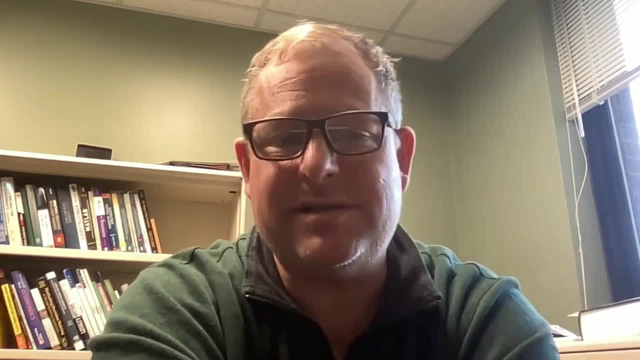 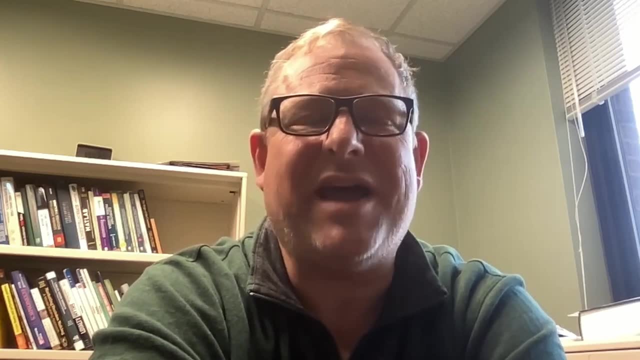 points in that process that create interesting research questions and interesting hypotheses that you can test. But absolutely I mean you've got to, you've got to be in there, You got to experience it, You've got to see it. And for my marketing students, one of the things we 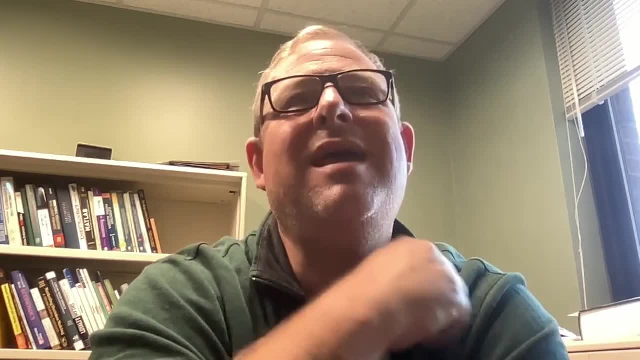 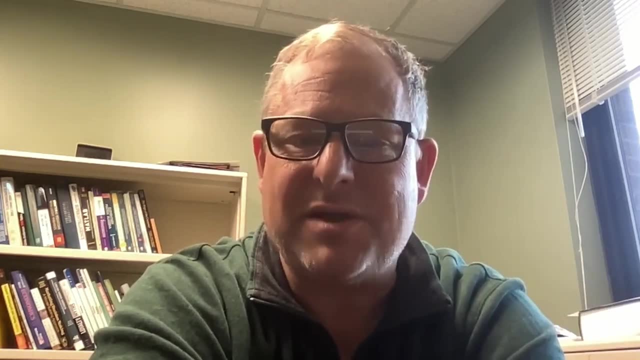 encourage them to do is not only have an internship but also partake in research. that will help them better understand business problems, not just, you know, more abstract kinds of questions when it comes to marketing, and being in the customer service environment is really a part of 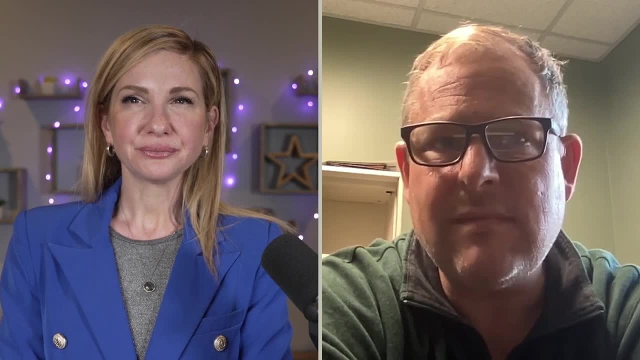 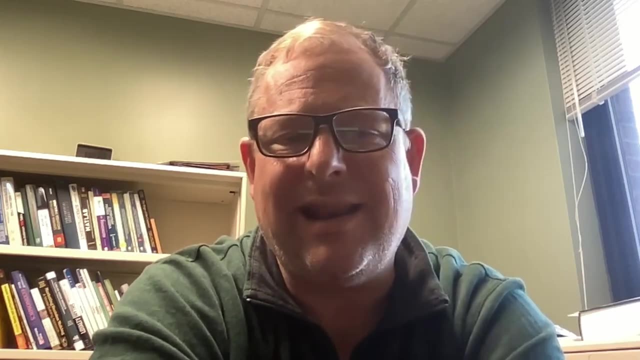 that. So you see it as a growth industry? I think so, Absolutely Right. I mean, we're going to. we're calling it different things now, Right, We're calling it business analytics and data science, And we have data scientists popping up everywhere, And they're the same people who. 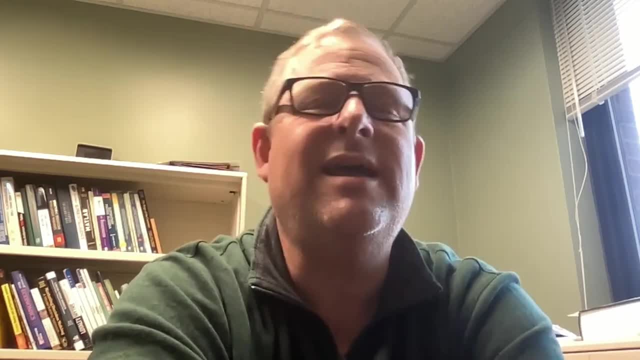 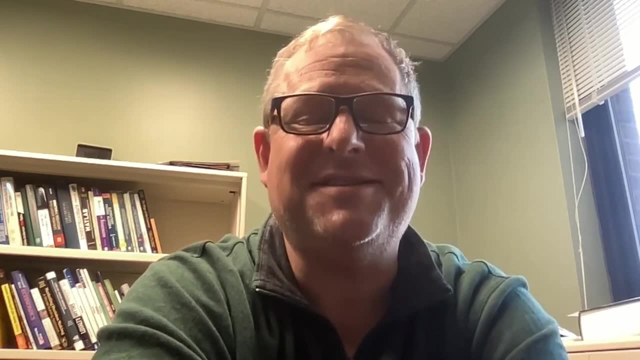 were marketing researchers 10 years ago but now they're data scientists. It really is one of the hotter job prospects. I mean, if you have the ability to to do rigorous analysis of data to better understand business problems, it's really an important tool that a lot of businesses need. 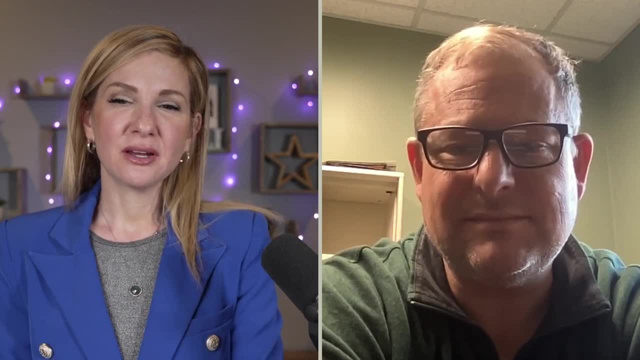 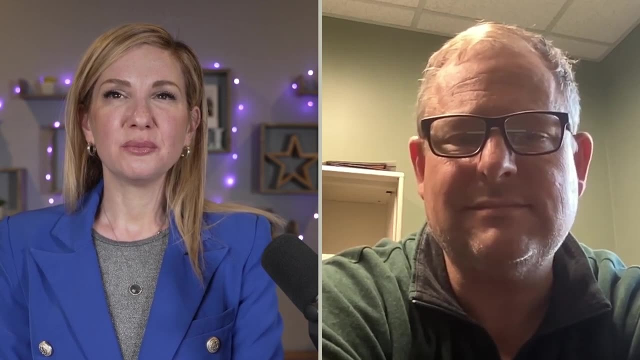 Well, I think it's a very exciting pursuit And I am so glad that I landed in customer service and customer experience. And I think it's a very exciting pursuit And I am so glad that I landed in customer service and customer experience. Well, let's get to know you a little bit better. 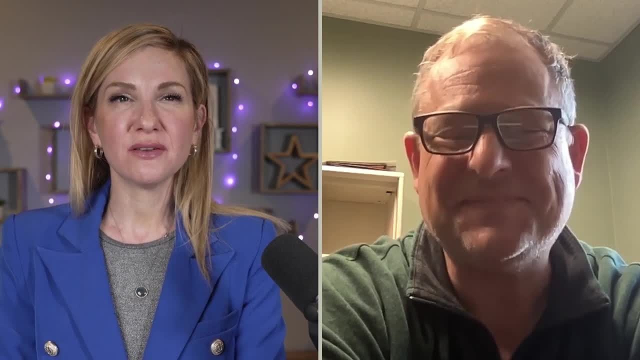 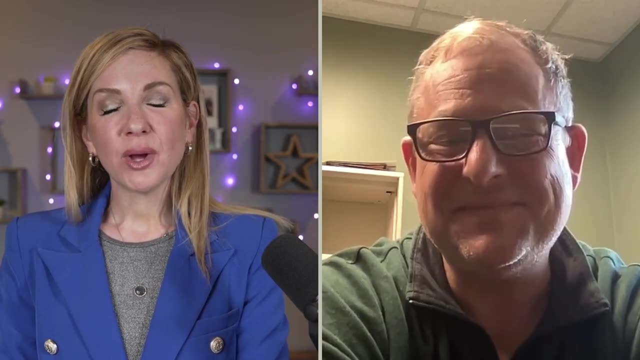 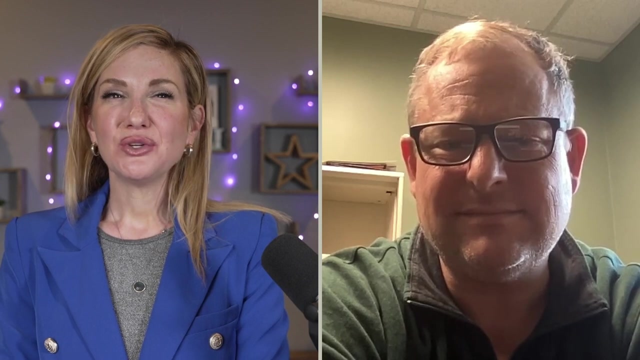 outside of your work as a professor and a researcher. Are you ready for some rapid fire questions? I will try, You'll try. That's all I can ask for. Okay, Number one: what is the most important part of your morning routine? Coffee, Same. Do you have a unique leadership hack that? 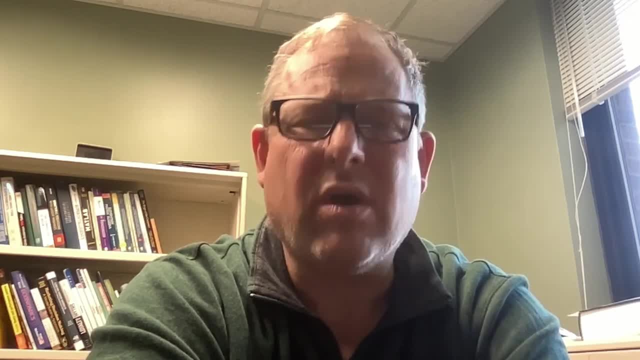 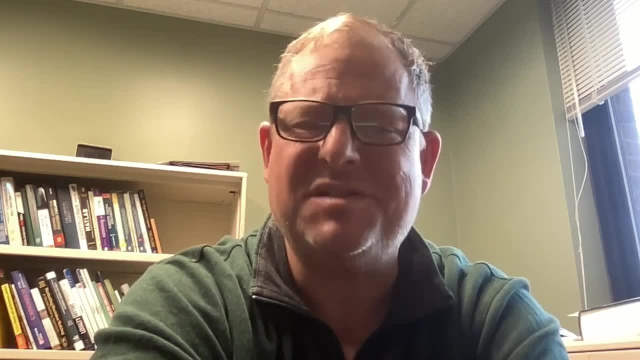 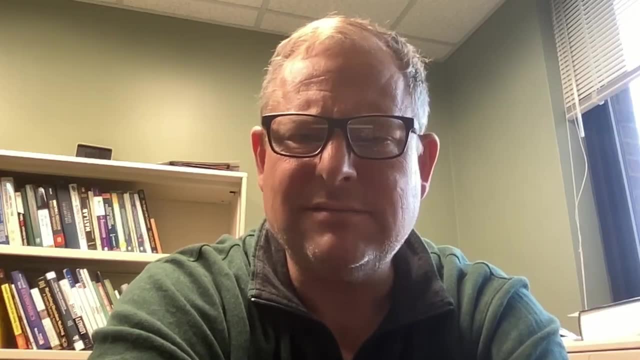 Using the people that work hardest in my life as an inspiration, source of inspiration to work even harder than them. What do you do to relax at the end of a hectic day? Nothing, Just transition into the evening. That's really it. I just transition into the evening. I don't know that there's any. 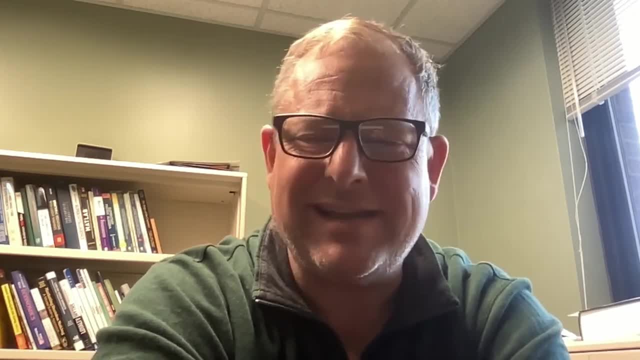 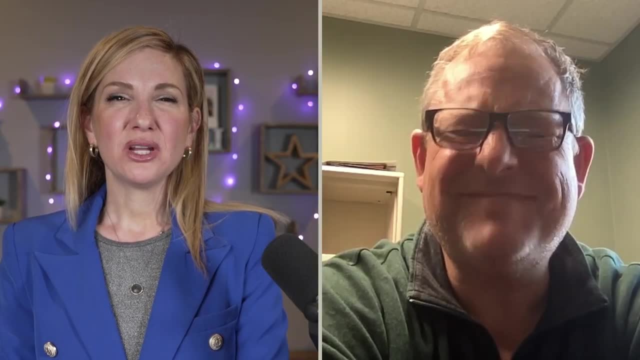 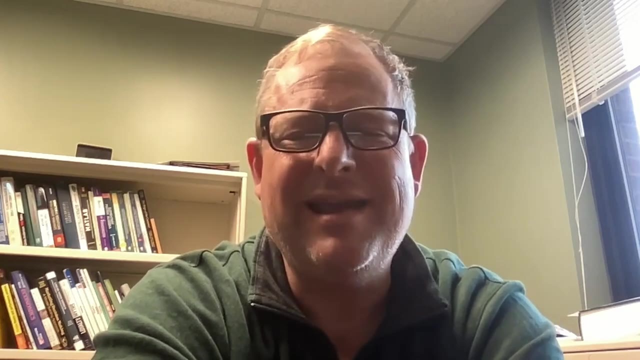 habit I have that takes me from the day to night- Okay, cool. What show are you currently streaming? None, Okay. What is your favorite leadership book or resource? Oh, goodness, Of course, I've got many, many books that I have read over the years that had 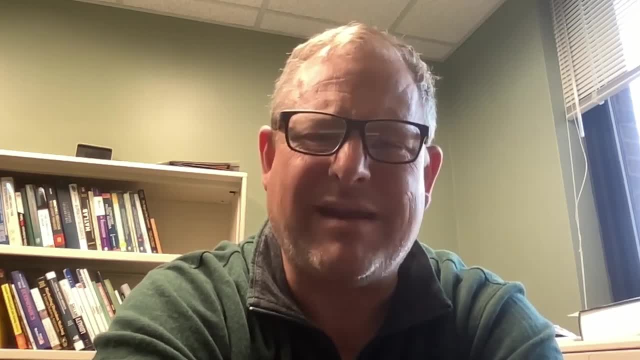 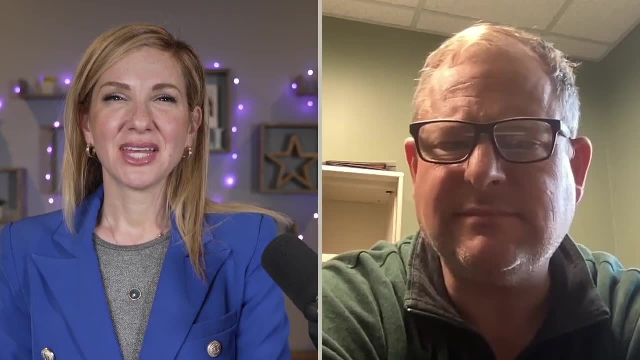 big impacts on me, but a leadership book in particular. I don't know if I have a good answer to that. Okay, What's your idea of perfect happiness? My kids and my family doing well? And if you had to describe your outlook in one quick motto, what would it be?